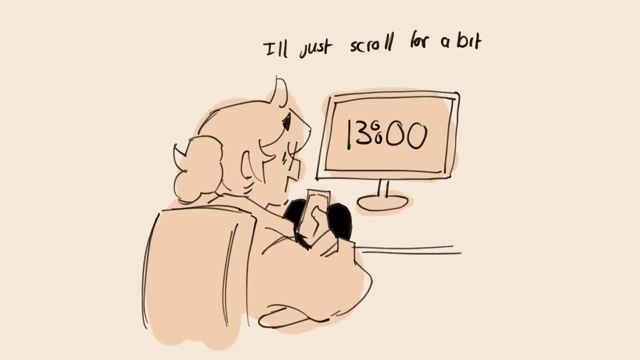 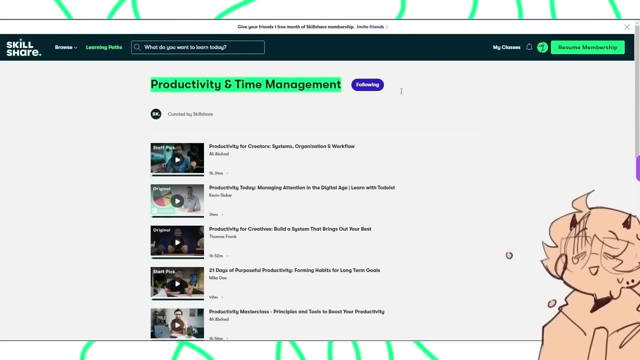 What I struggle with is I'm a heavy procrastinator and I find myself daydreaming more than I'm actually doing work, And I lose track of time, deadlines and projects. A class that gave me a lot of insight is a class called Productivity and Time Management. 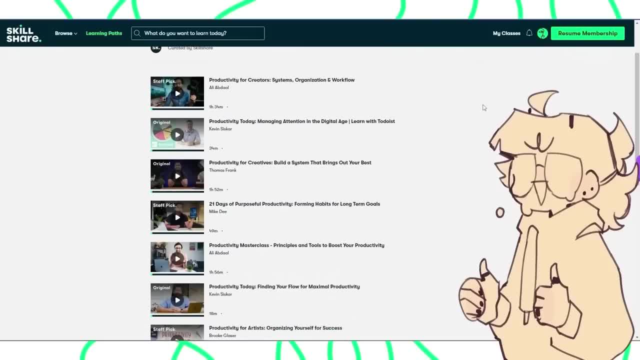 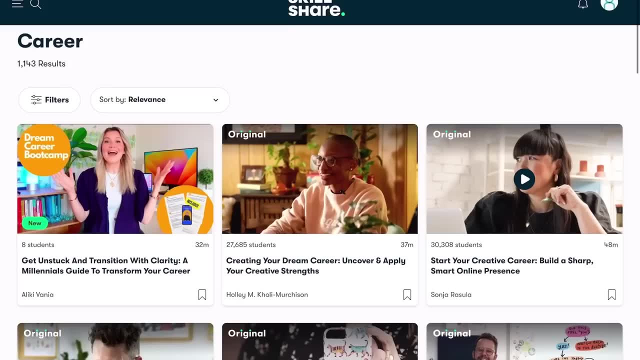 where I learned how to sort and manage projects I had to do, how to organize my schedule to fit me and how to build habits that stick. Now I'm only spending 25% of my time staring into the void. There are many more career-focused classes. 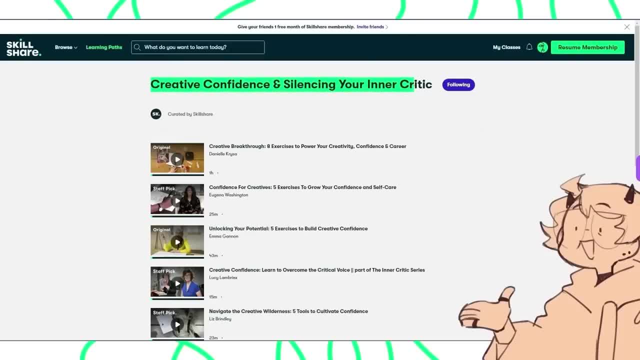 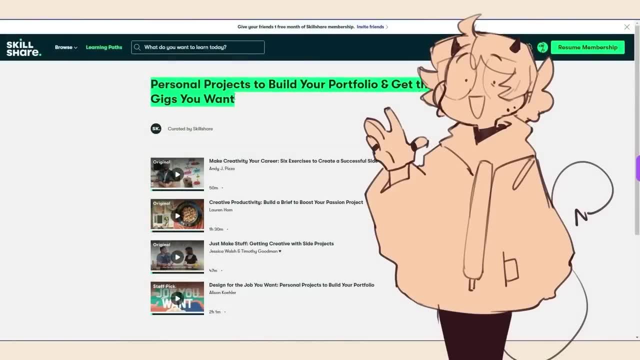 on all types of topics like creative confidence and silencing your inner critic. This one is a actually really eye-opening and i definitely recommend it if you struggle with this: personal projects to build your portfolio and get the gigs you want. build a creative career, full-time or 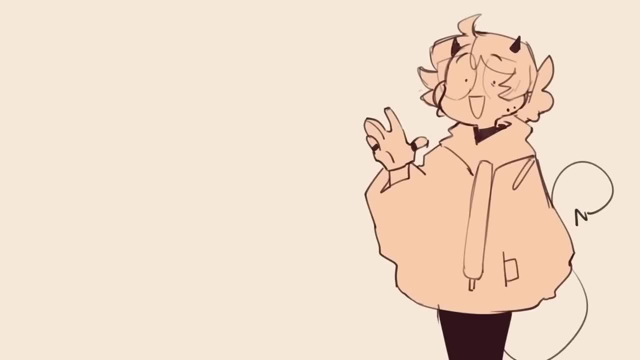 freelance and so many more. learning and developing is a great way to spend your time. so whether you want to build knowledge and how to build and manage your dream career, or learn fun and interesting hobbies, skillshare has classes covering all your interests. skillshare was kind enough to offer the 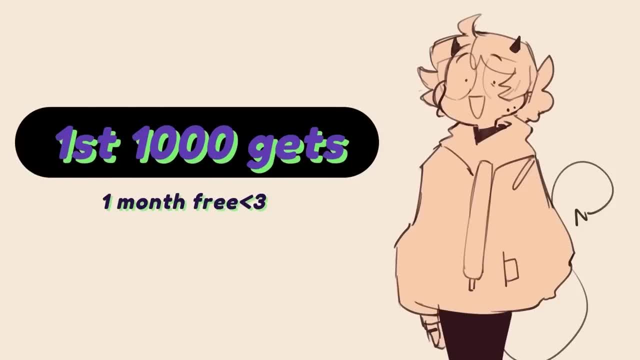 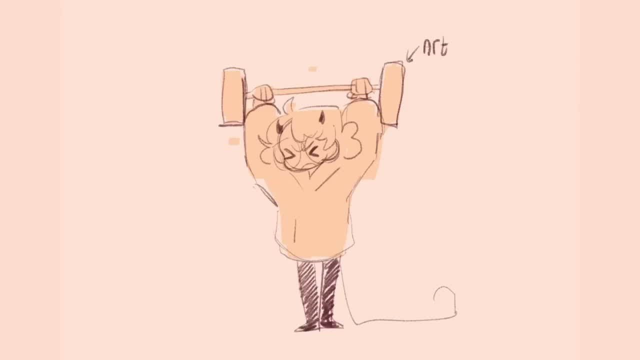 first thousand people to use my link in the description, we'll get a one month free. thank you again to skillshare, and now onto the video. being good at art is all about practice and studying until it becomes muscle memory. color is the same as any other art skill some artists have. 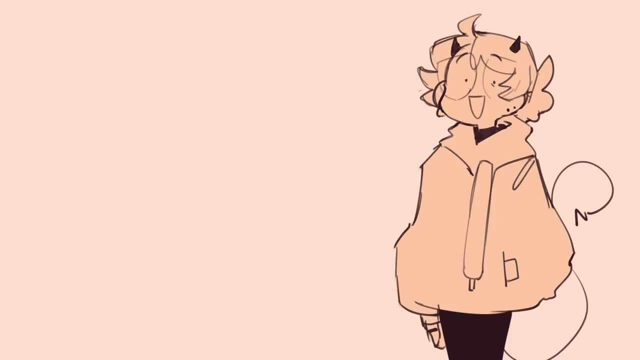 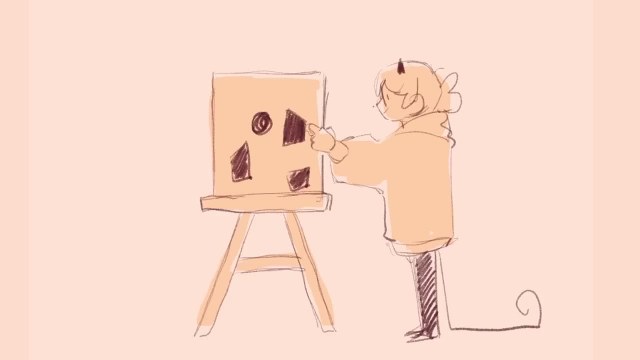 a natural eye for color, but you can only become truly good at it with trial and error. here's how you can study colors and get better at picking them for your pieces: simply just join them from other artists. i don't mean just outright steal their color palettes and layouts, but color picking 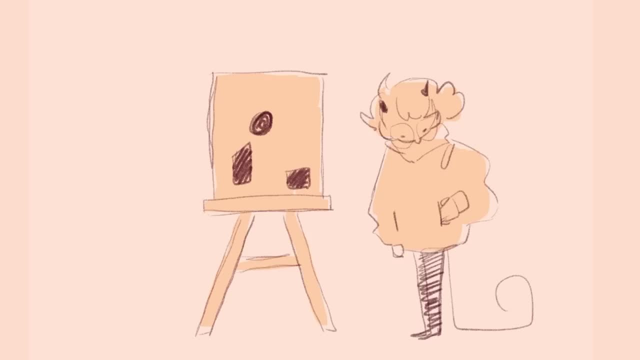 and do color studies with these artist pieces that you really like. like laying out the color palettes and layouts and doing color studies with these artist pieces that you really like, colors on a canvas and observing where the artists use and saturation, mainly on the color wheel. can. 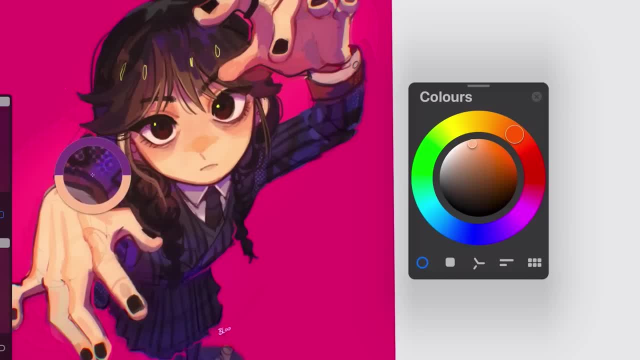 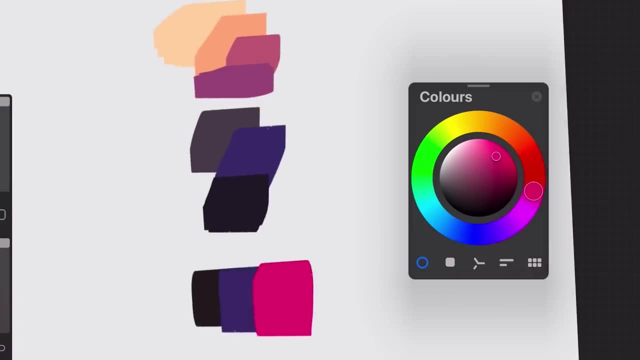 give you good insight on how they pick colors or why the colors work so well. pay attention to where the color wheel goes as you hover over the colors. add the same colors to a piece and see if you can create the same effect. play around and see what you can add to improve it, for example, adding more. 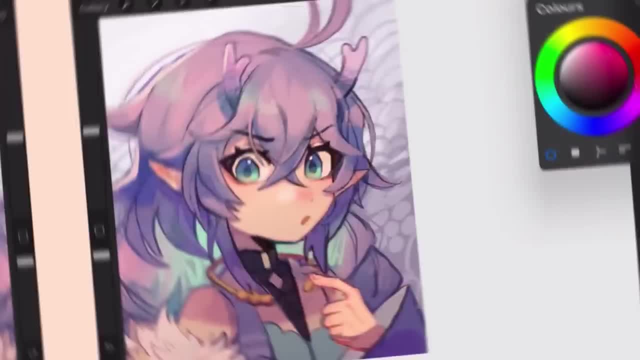 values or heighten the saturation or lower the saturation. another way to get better at color picking is not to use the color picker when you're studying an artist thing, but try and find that color on the color wheel. you can use the color picker when you're studying an artist thing, but try and find that color on the color. 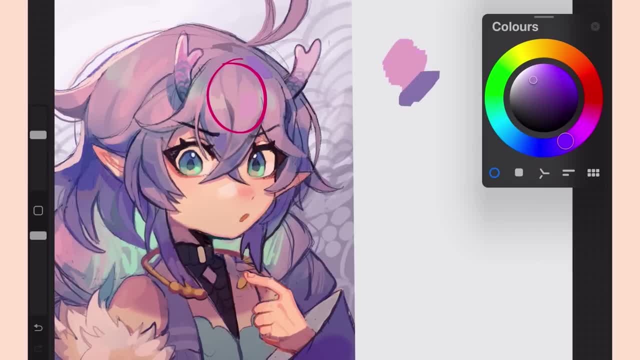 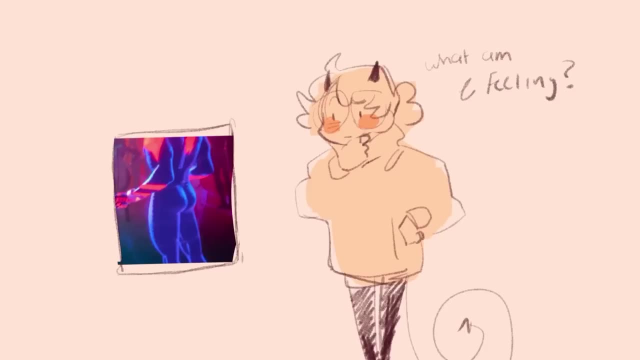 wheel. you can use the color picker when you're studying an artist thing, but try and find that color on the color wheel. this will give you a really good understanding of color context and how colors interact with each other and where to find these colors on the color wheel. another thing to study is how this piece makes you feel. what about this? 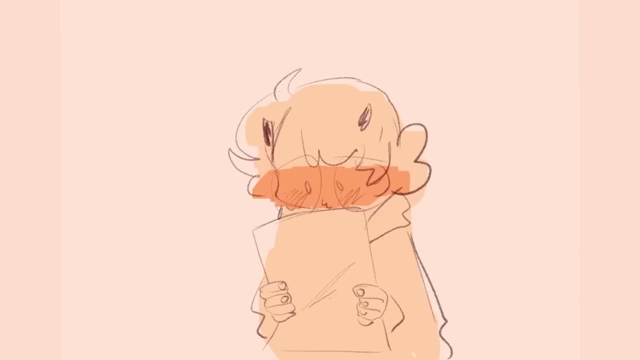 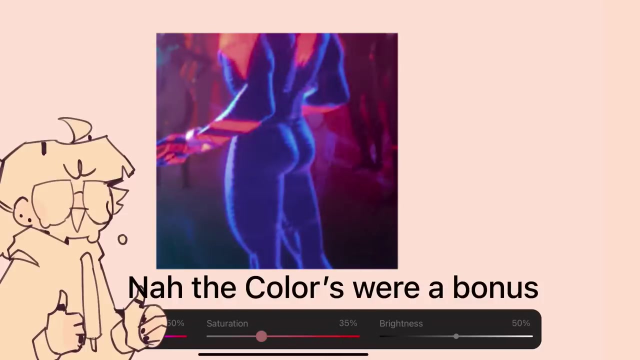 piece makes you feel that way? is it the colors, the values, the saturation? is it the layout? take away the colors and see if the piece still feels the same or if the colors had a big impact on the atmosphere. look at which of the area of pieces catches your eye and why that might be. make notes. 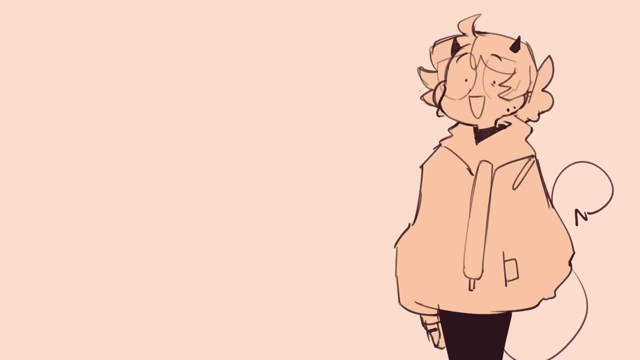 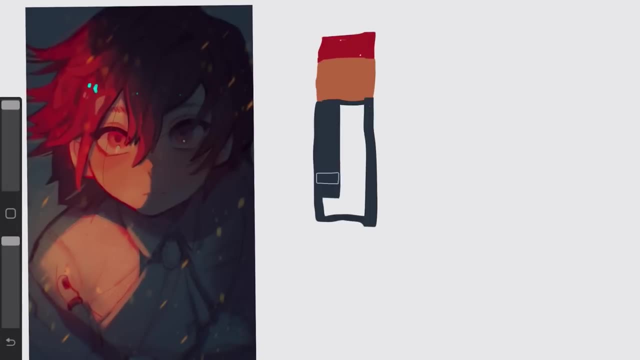 and see how you can add this to your work. study color palettes as well. which color scheme do the artist use? try and figure out which colors they use as a primary and which color the colors they use as a secondary. when you pay attention to the color choices of other artists, it becomes a lot. 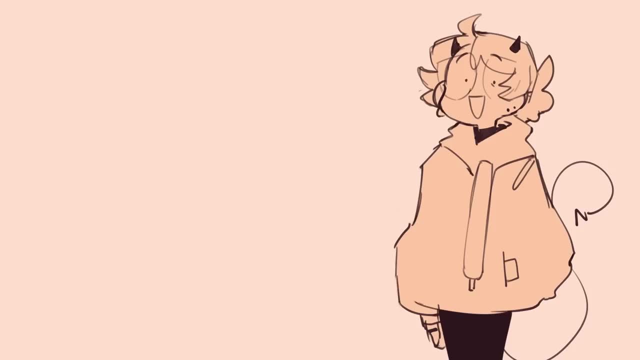 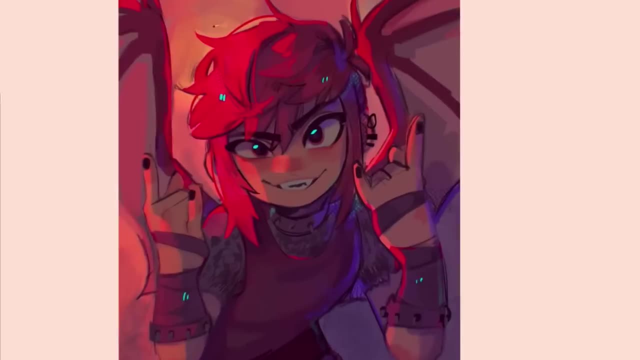 easier to pull the knowledge of color theory up for yourself. composition doesn't just come out from the layout or the drawing. colors and values play a big part in the piece coming together and the piece having a focus point. a focus point is a place where the viewer's eyes will rest or move. 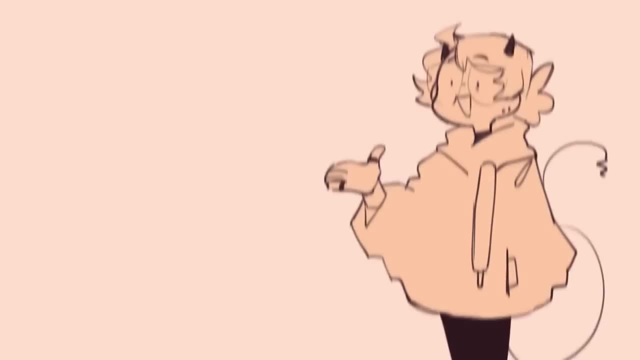 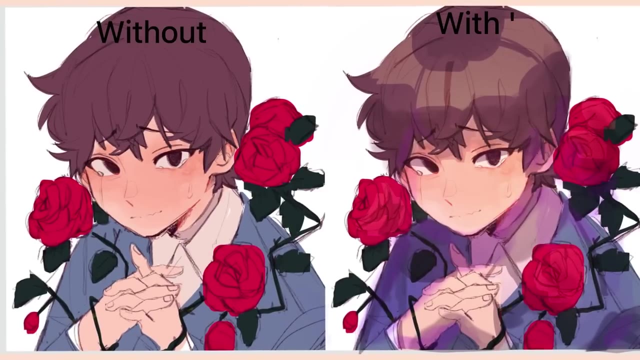 towards values and lightings play a huge part in picking colors and laying them out. without differing values, a piece can look flat even if the colors are beautiful. values adds depth and you work creating a piece that is nice to look at. although a flat colored art style can look, 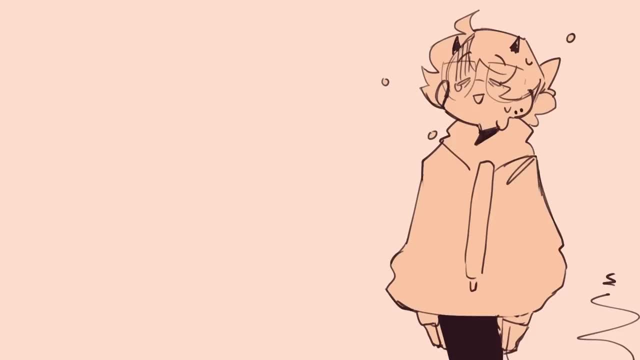 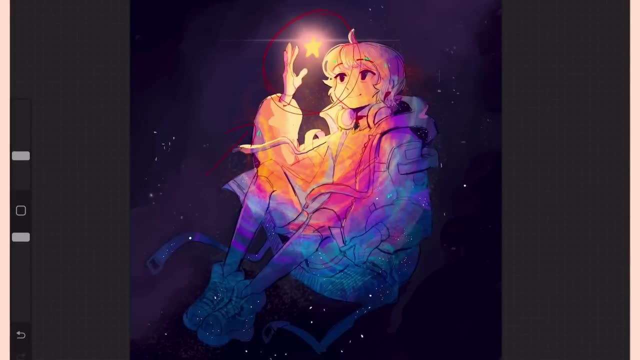 amazing if you have the skills to pull it off. but i'm talking about my style today and how i pick colors and i value a lot of values. i guess generally the brightest area of pieces where you want to draw, the eyes will naturally fall and then trail towards the darkest. using the 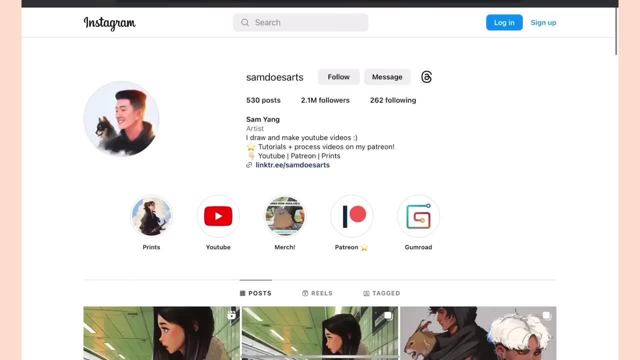 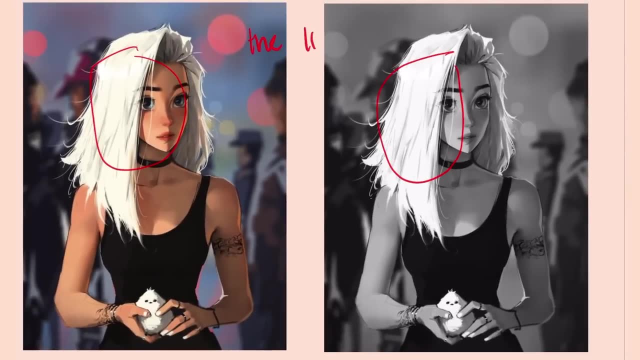 information. you can make the viewer look and pay attention to where you want them to, for example, sanders art. he's very good at drawing attention to areas he wants the viewer to look, which are the faces of his characters. they're highlighted with brighter colors, which naturally draws your 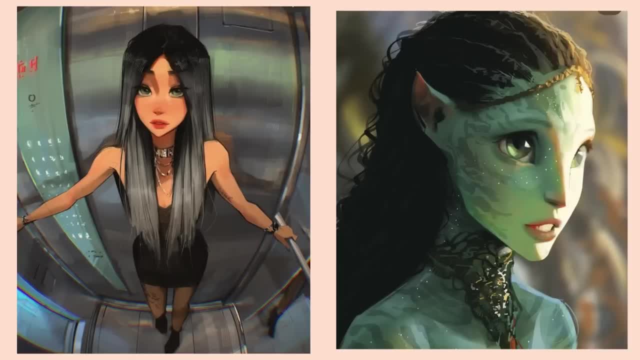 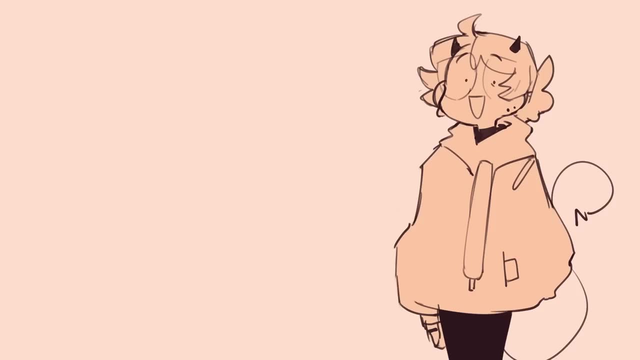 eyes towards them. along with his very pretty style, it works very well. making a piece gray scale first and laying out the colors to figure out where the lightest values should go and the darkest, can make this easy. a place where you want the lightest values to go, so where you want the viewer to look, and then plan. 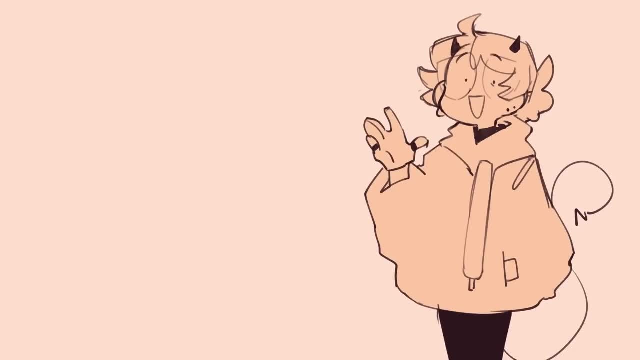 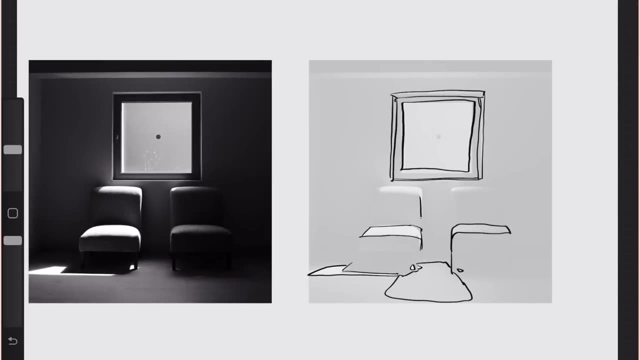 it out like that. a good way to practice values and lighting is to do photo studies, where you pay attention to the lightest part and try carving out an image using black and whites. this is a little tricky at first, but it helps our eyes to build figures using values alone which, once you learn, 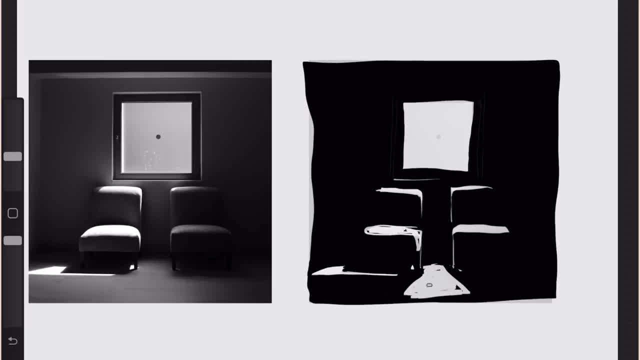 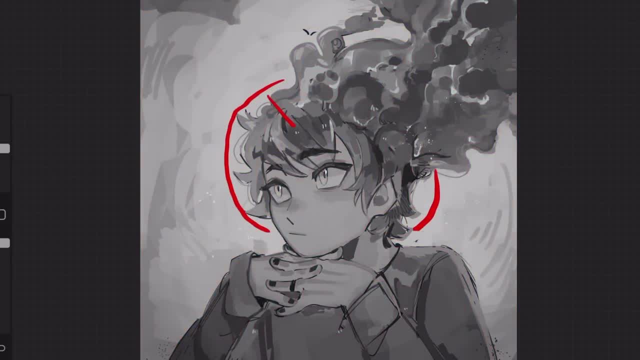 this, we will be able to build figures with values alone, making the color laying out process a lot easier. in this piece, if i turn on the gray scale, the lightest area is the background. the lightest area is the background, that is, the back and the bottom, where the lightest color is going to be. 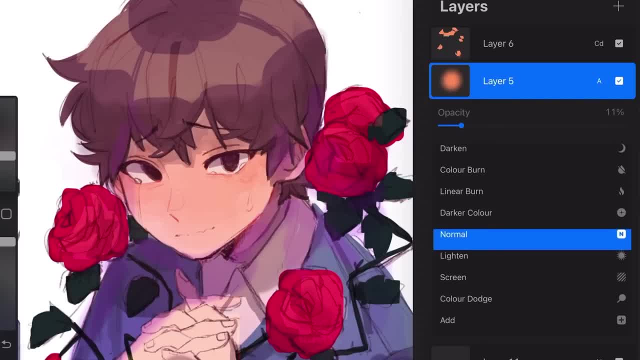 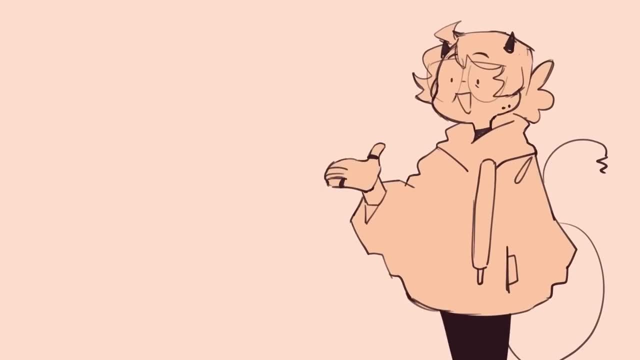 so i will try to plan out the colors and values using the gray scale and then i'm going to apply the gray scale to the edges of the face so that i can create a little more contrast to the edges. i'm going to focus on the eyes of the face and then i'm going to apply the gray scale on the. 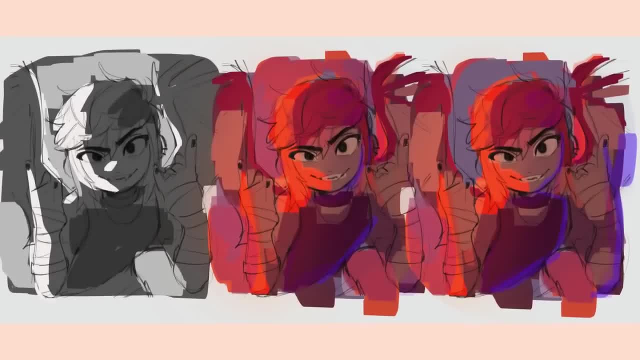 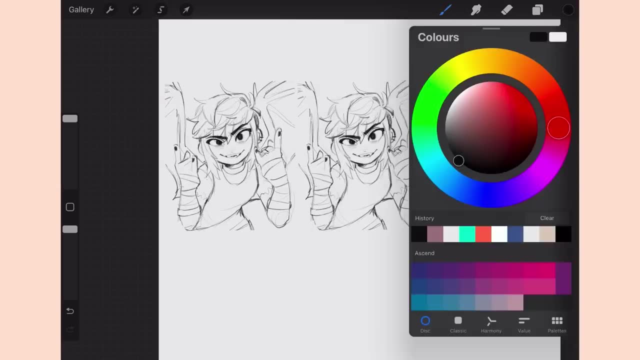 top of the face so that my face is a little bit more transparent and more visible to the people. while highlighting his face, which brings your eyes to the focus point and which will trail off further, then i love highlighting the face with an overlay layer, since the faces are what i want people to pay. 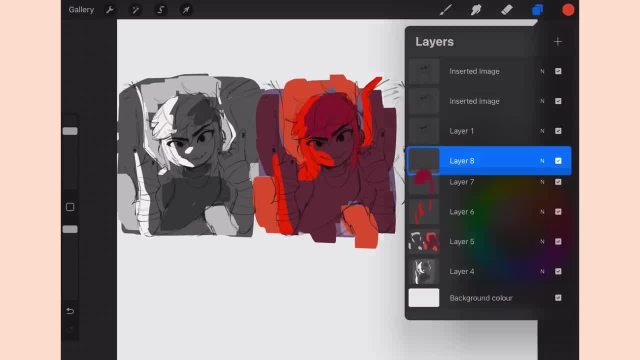 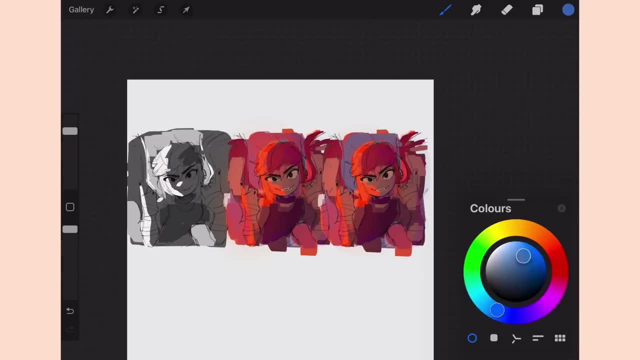 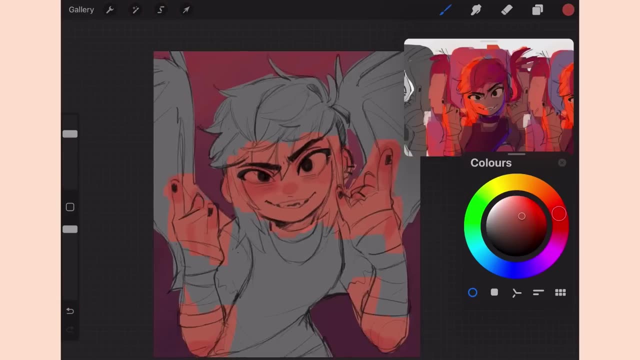 lot smaller and start messily planning out the colors and values, doing different colors, different palettes to see which one I like more. Once I have that done and I'm happy with it, I copy paste it into the corner of my art piece and then add those colors to my piece. This makes it a lot easier and it's also a lot. 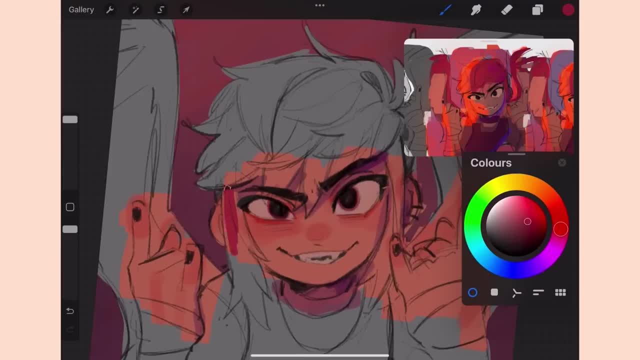 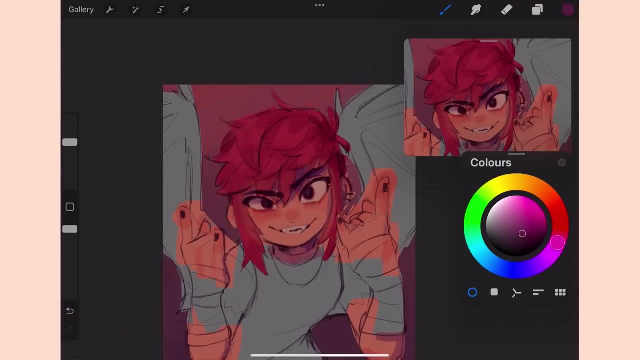 easier to add colors to a smaller drawing, so I think this is really helpful to speed up the process a little bit and it also eliminates that one of like I've done this entire color palette, I don't like it and I have to start again. Before we get to the color picking side of this video. I did color color. 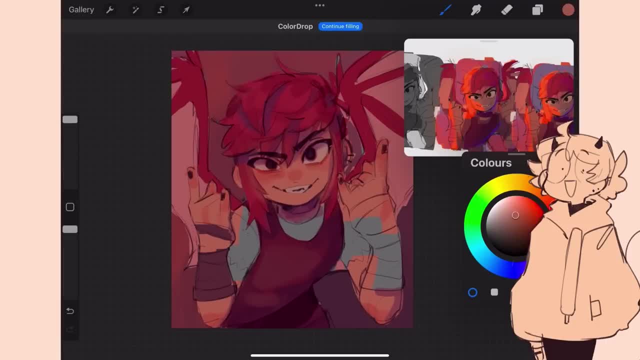 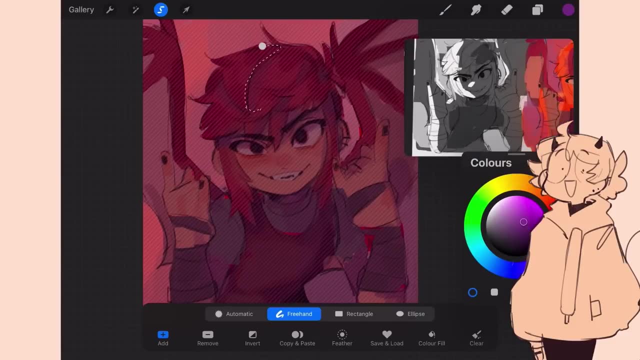 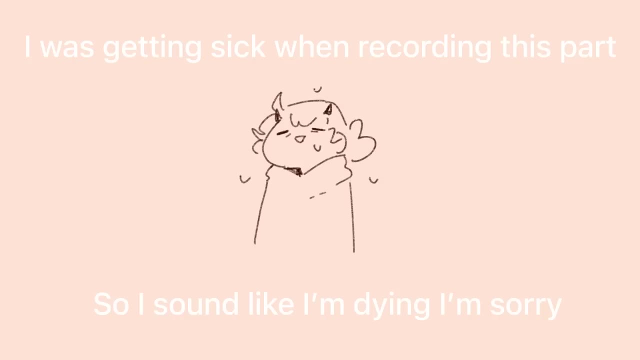 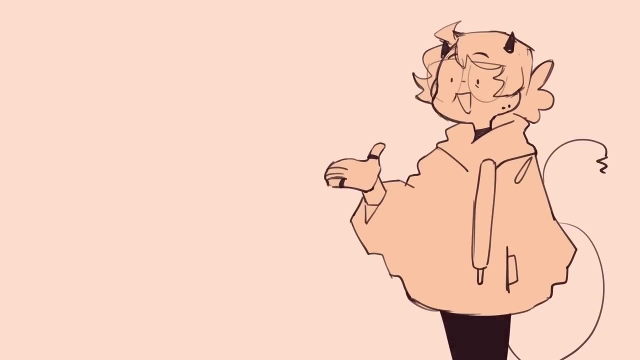 schemes and color palettes in my last video about color theories- and that is very important. I really suggest looking at that and doing your own studies on that, because that's not something I can explain too well, so just make sure to go check that out. I make use of basic color theory and observations on what looks nice when I'm 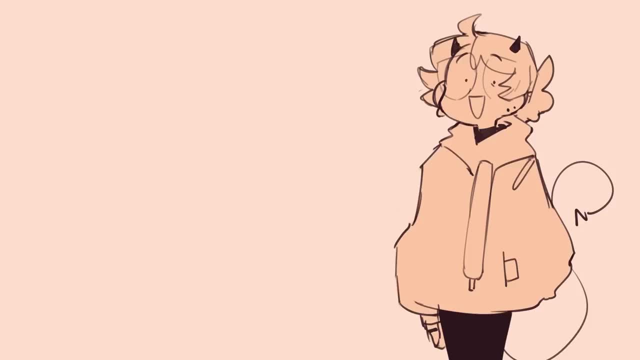 making color choices. A lot of my knowledge has been built up from observing and studying how other artists pick and layout colors and their use of values, Like the study methods I pointed out at the start of the video. So first I kind of have an idea of what color palette I'll be using or which hue I'll. 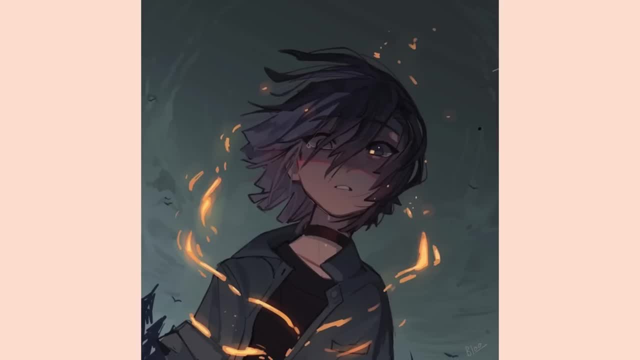 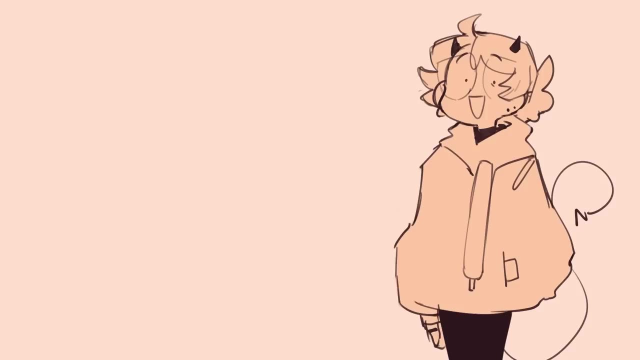 be sticking with. Keep in mind, the atmosphere of the piece is a dark, happy, sad, and which colors suit that kind of atmosphere? Planning out these is all up to you and your art piece and what kind of like piece you'd like to go for. But that's why I mentioned that studying 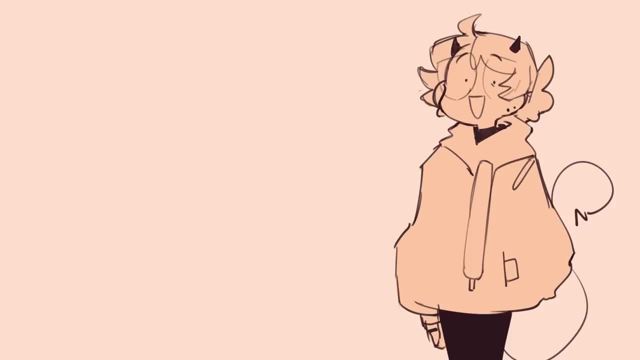 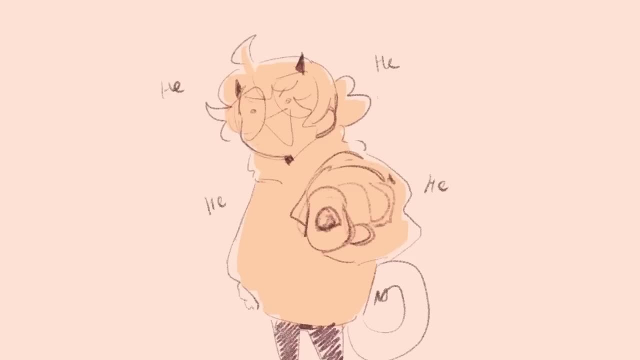 like color theory, atmosphere, which colors connect to which mood, and all the stuff is very important. So it's all up to you, since art is a creative medium and I can't tell you which colors to choose for your piece. It's up to your. 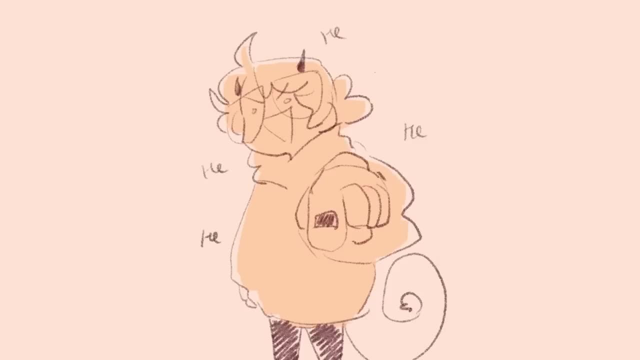 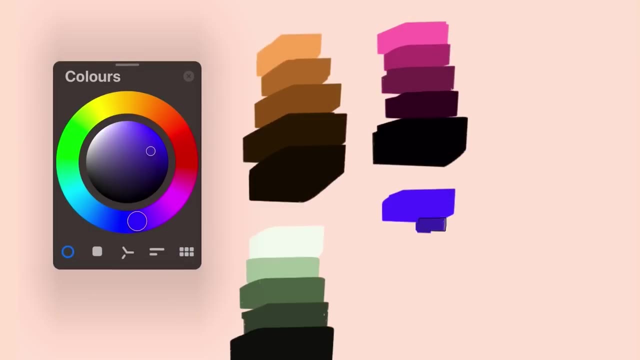 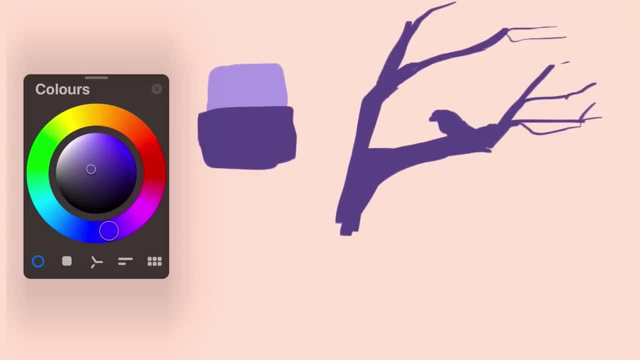 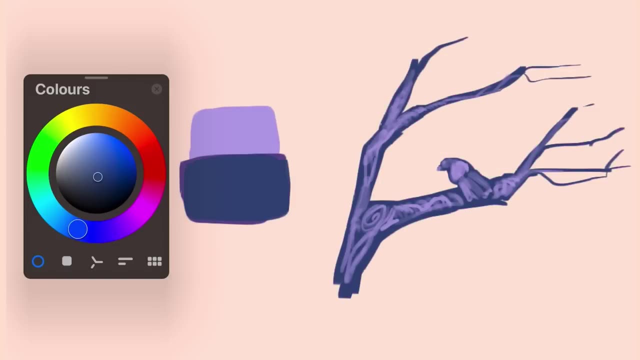 purple. Just using these two I can carve out a figure. I'm using monochromatic color palette to do this. You can shift the darkest hue to a different value and it'll still be the same due to the values. So this is called an analogous. 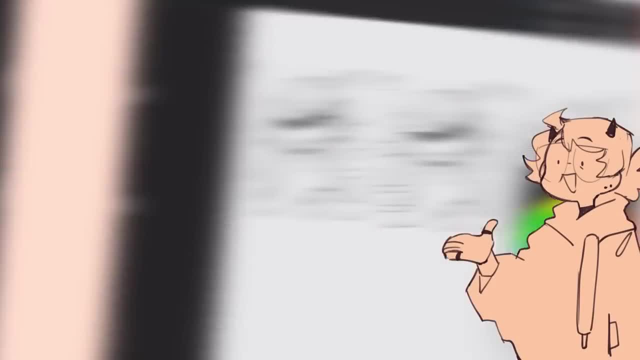 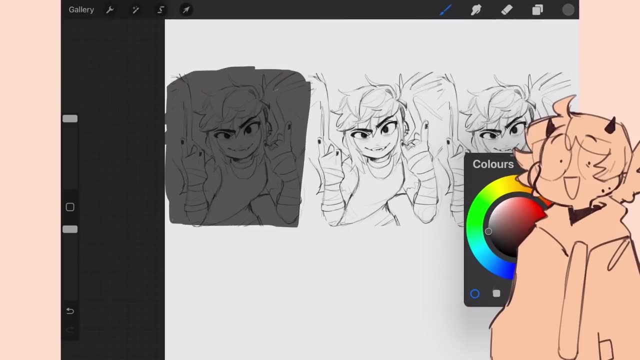 color palette because it has two or more hues in it. When I'm like planning out my piece, I already have an idea of where I want the lightest piece to go and then the darkest. Again, you can use the thumb nailing process to be able to plan this. 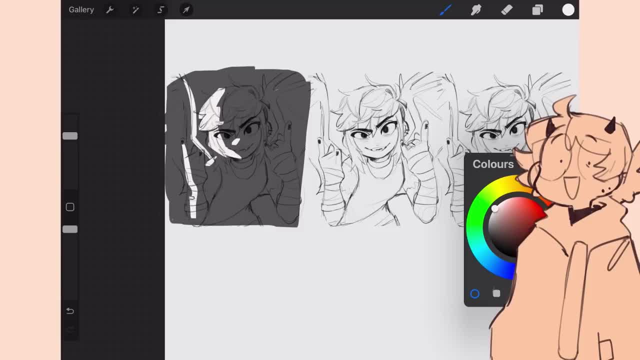 out like I showed you with the Nimono piece. So this is a really useful. it helps a lot with the planning and makes it a lot easier and it eliminates a lot more mistakes, because sometimes when you're going in and you're laying out the colors, you can make mistakes like: oh, I realized this part is not dark enough. 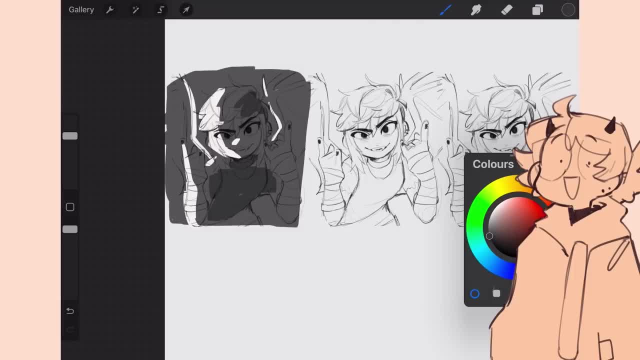 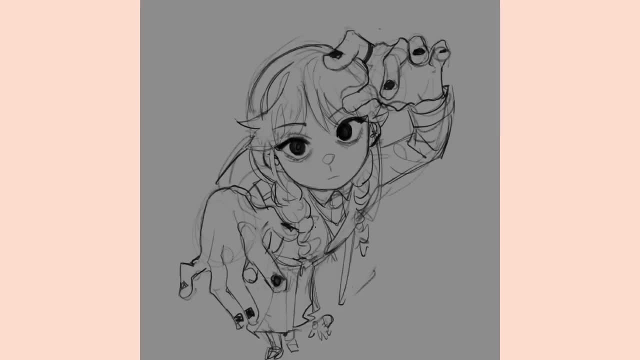 this wasn't light enough, then you have to go in and change it. So the big part of where my colorful art style comes from is the shading, lighting and random colors I throw into a piece Once the base colors have been laid out. it's a. 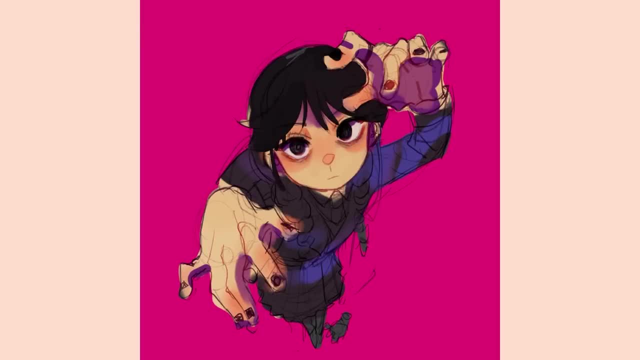 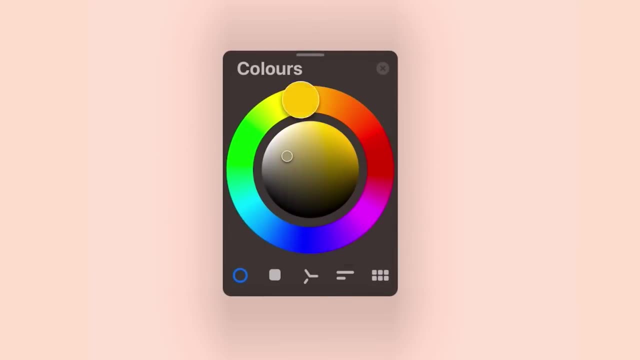 lot easier to start picking the colors that really make the piece pop and give it that depth and color. The color wheel is your best friend when it comes to picking colors. the way it's been laid out makes it a lot easier to be able to find colors that harmonize with each other. I covered the color wheel. 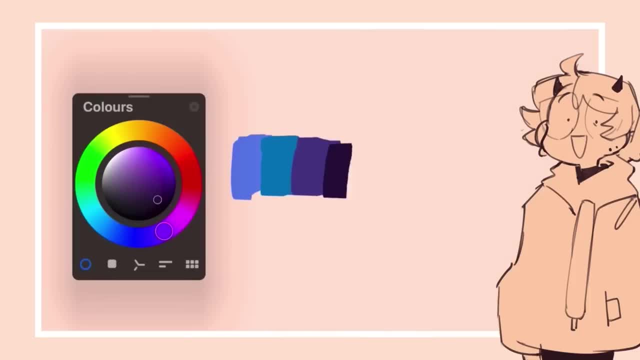 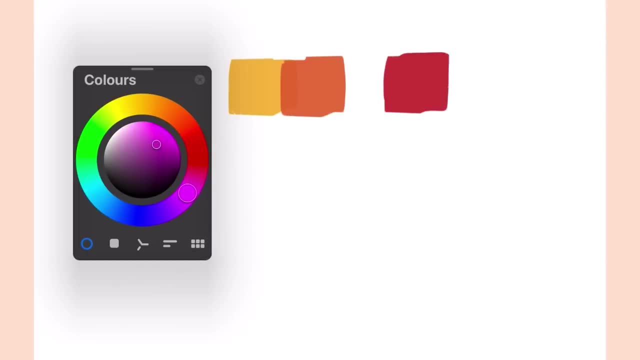 and how you can find color palettes that work with each other in the previous video. so I won't cover that in this video, but I will go over how I kind of use it now. So for me, colors that harmonize with each other are colors that look. 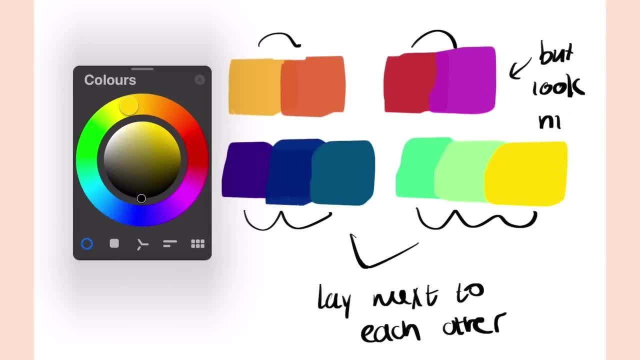 really good. For me, those are the colors that lay right next to each other on the color wheel, So orange is harmonizing colors with a hue shifted down a notch on the color wheel, So it's either a dark or a light color, Or it's a dark color with a 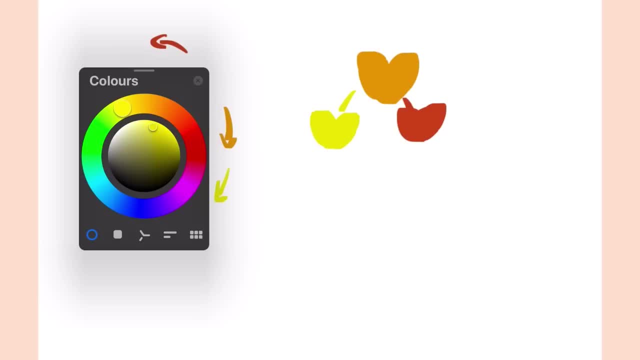 yellow or this red, And then another shift down for a more harmonizing color. so then it's like either this pink or this green. So that's how I use the color wheel to find color harmonizing colors, because it's basically just the colors that are right next to each other. So when I'm shading, this is what I do. If 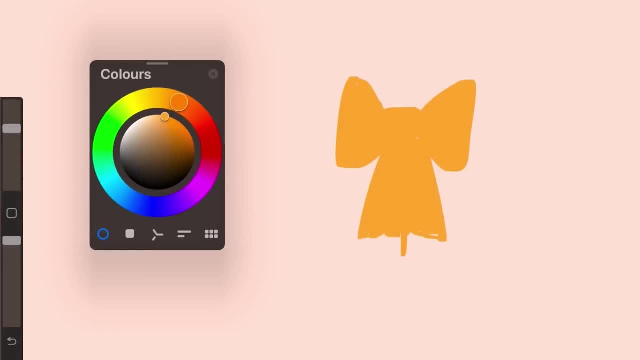 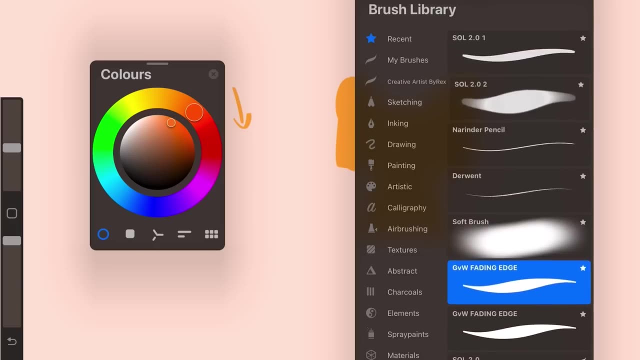 the base color is orange, I will shift the hue to the color right next to it. I'll shift down the saturation and then I'll lay that on to the base color for a shading. I really love shading with purples and blues, so I shift the hue towards the colors that are closer to blues and purples. 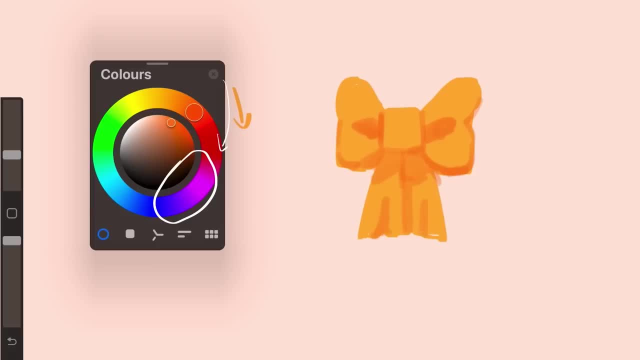 That's why I go towards red and pink instead of green and yellow for the orange color, because I wanted to lean more to the colder, more pink, purple kind of colors. You can keep adding this, so rather than just one hue shift down, you can go another one and another one, depending on like the base color or what. 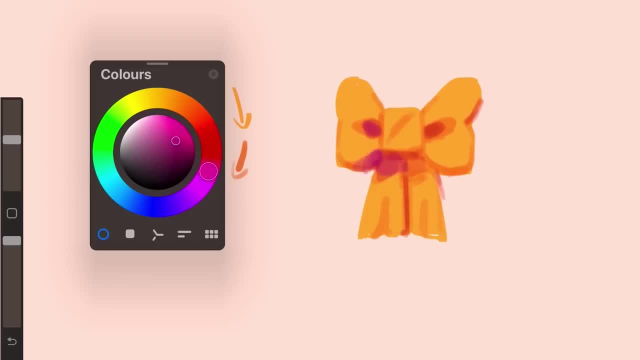 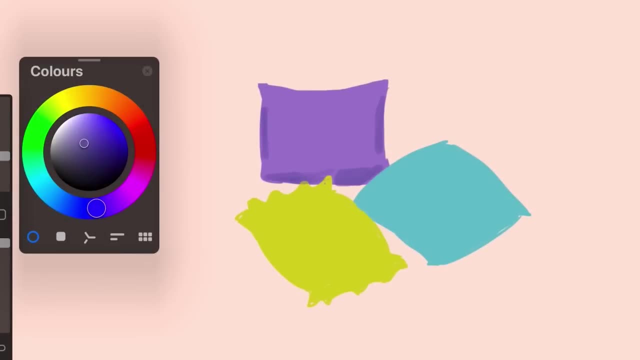 you are shading. If you want more shading colors, you can keep shifting. keep shifting, like with the hues and the saturations. Once you understand this, you can go down to red. you'll be able to make vibrant shading colors. it's the basics of what I do when 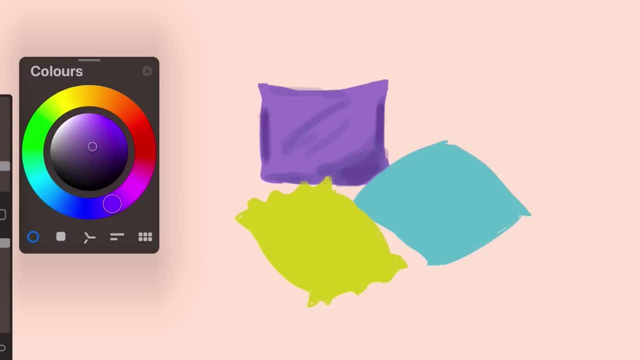 I pick shading colors, for example, of three different base colors. if I add the shading to them, I'll use the color wheel, pick the base color and shift the saturation to a darker value, and then I'll shift the hue to a hue just next to it, but I'll shift it towards the purple or the pink. so this will be the shading. 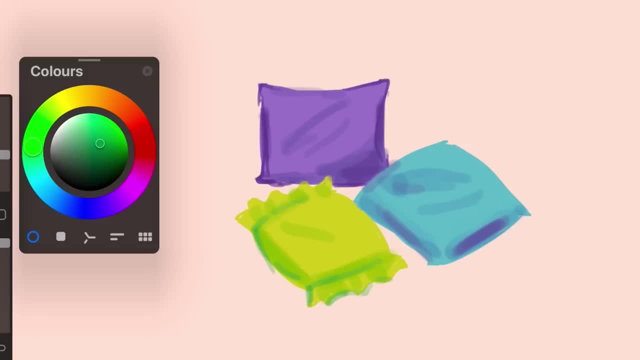 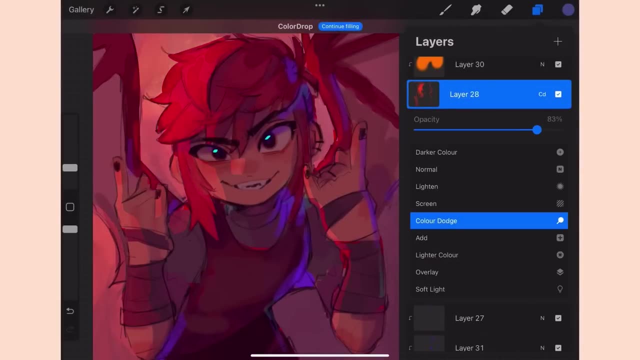 color if I want to add more shading colors by shifting the hue and saturation to the color just next to the one I just picked. remember colors next to each other harmonize. I make use of the color opacity a lot while I'm laying out colors for shading. it makes the colors I lay out mix with the base color a lot. 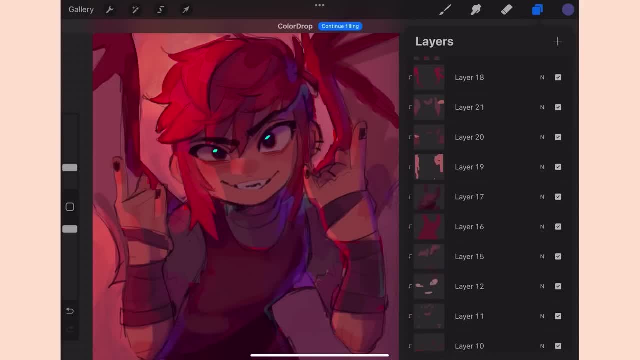 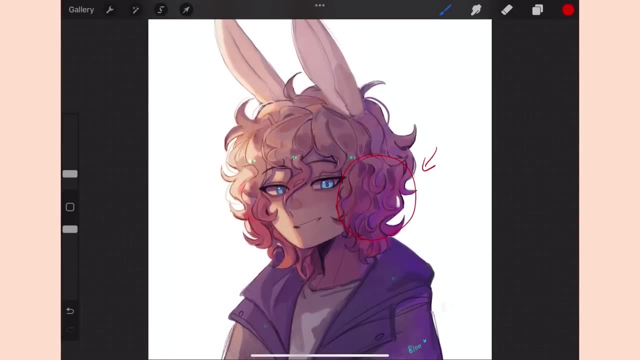 more so. if a color is too dark, I'll apply it to the drawing and then lower the opacity of the layer till it suits it well. a second layer I always add is what I call a far away color. I add it to the areas that are the 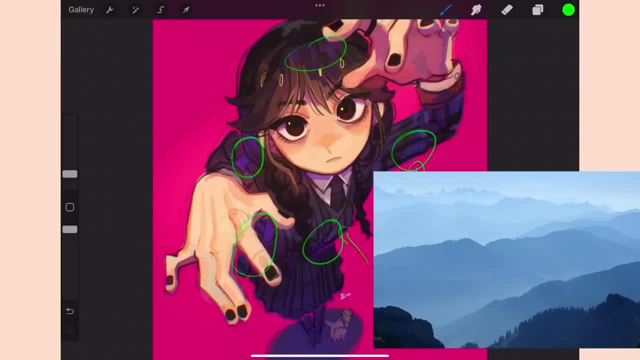 darkest or the furthest away from the viewer, kind of like when you look at the mountain in the distance. it's like this light blue color, except I use purple and turn down the a little bit of the color and then I add a little bit of the color to the. 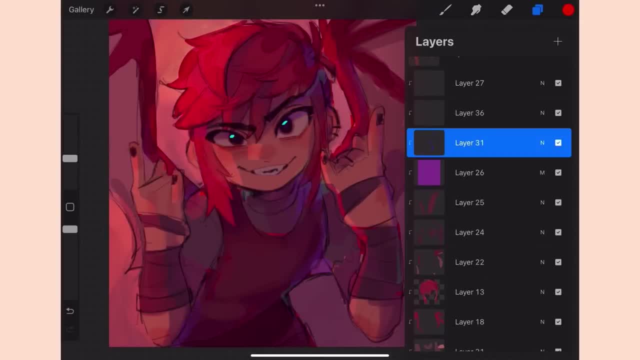 layer opacity. this suits very well since, remember, I shift the hues towards the purple or the blues or the pinks anyways. so adding this little bit of extra, like more saturated purple, just helps it pop a lot more. so something else I'd like to touch on is gradients. I've been using gradients in my work for a very long. 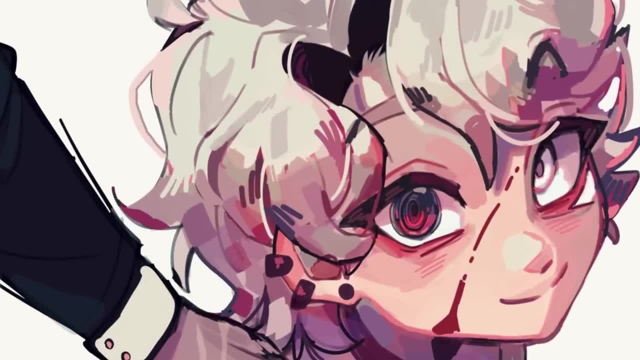 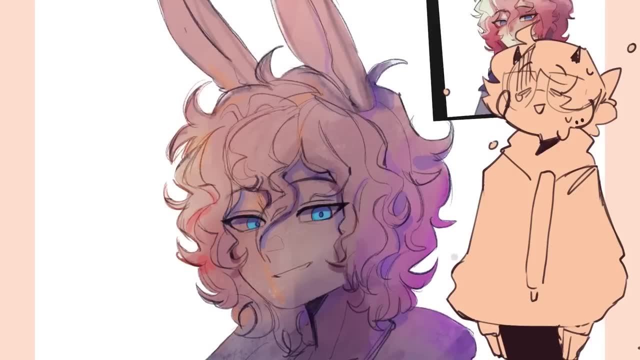 time because I have a very painty style. I love when colors bleed into each other and give a great, almost blended look to them once I paint them. just be aware that if you're not using a painting style and you do this, it can make the colors look really muddy and a 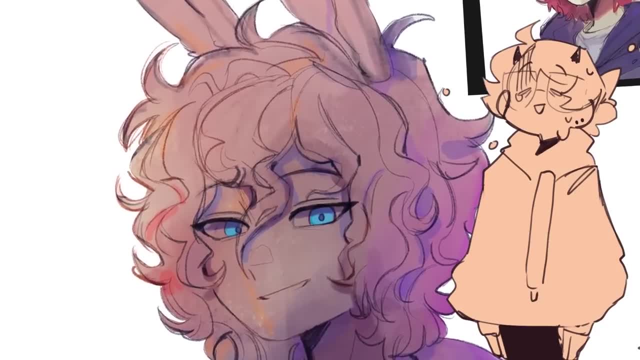 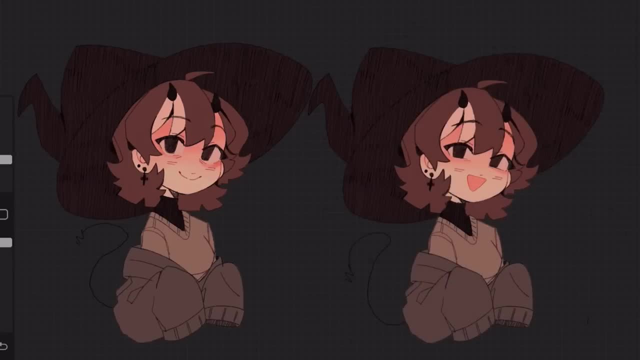 really blended it into each other, so I don't use this everywhere, but I use it on, like, certain areas. so I do this a lot with the hair and skin tones. for example, once the base color for both have been laid out, I will use the airbrush color. 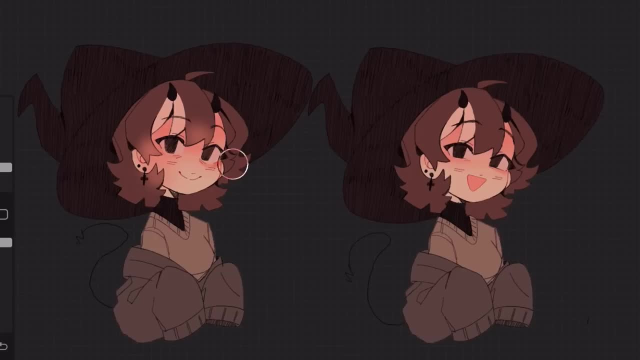 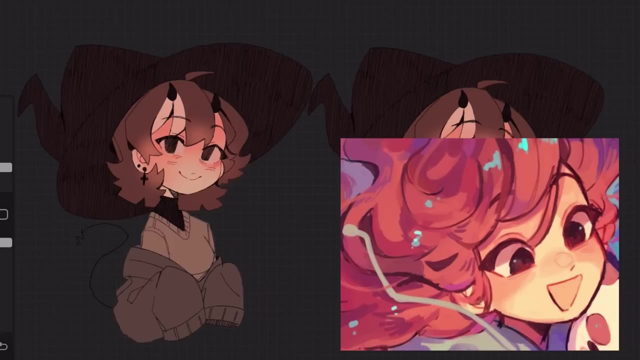 pick the skin tone, so the pinkish red, and then I'll add that to the hair where the hair makes contact with the skin, and once I paint that it kind of gives it like this softer look around the face. I do this with clothes as well as wherever. 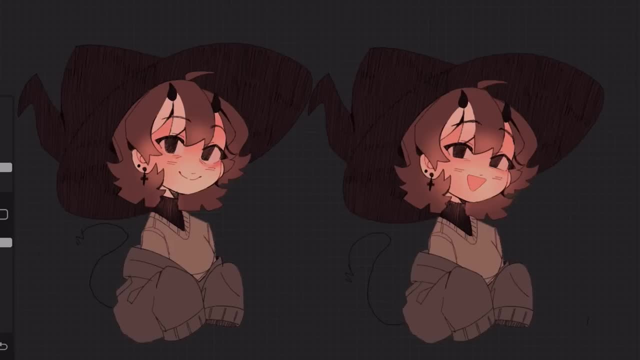 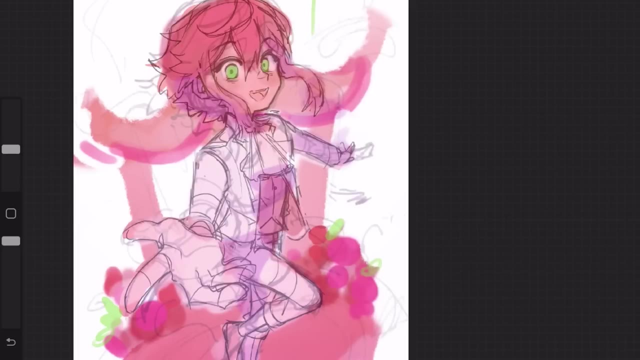 the skin makes contact with. I get dark clothes. I'll add that they're the same we shadows and lightings. when I lay out the colors, I do it very messily. I think that's very obvious and kind of all over the place, not really caring too much of. 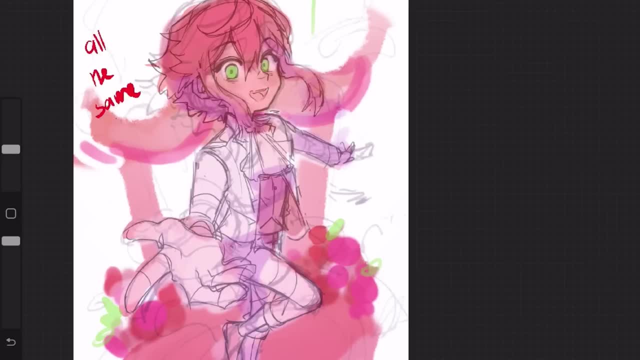 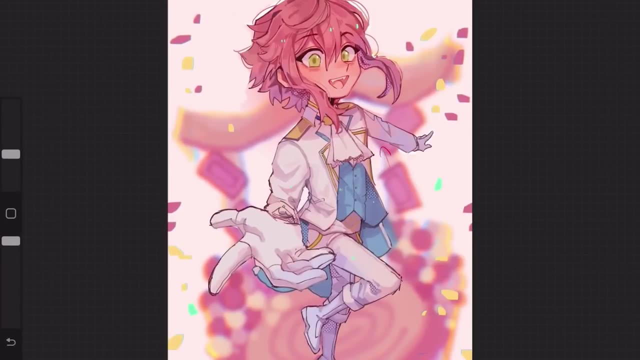 it the line work and then I turn them the layer opacity to create a gradient look between the colors. so when I add the purple that I was talking about, I like lazily, kind of was put it all over the place and then I'll turn them layer. 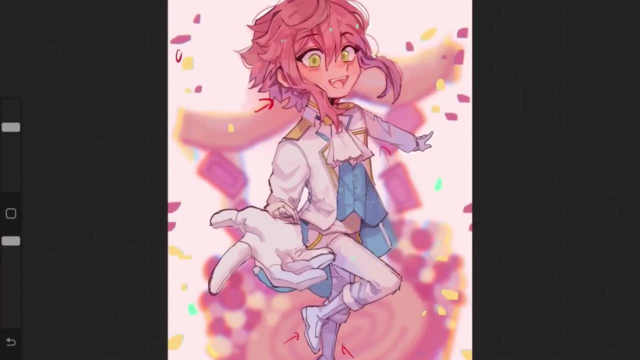 opacity. turning that layer opacity will make the colors that are underneath blend together. but adding the same purple on top of everything will make it like blend kind of together, since they're all kind in the same hue since the purple have been added. it's a little bit hard to explain, but it's better if. 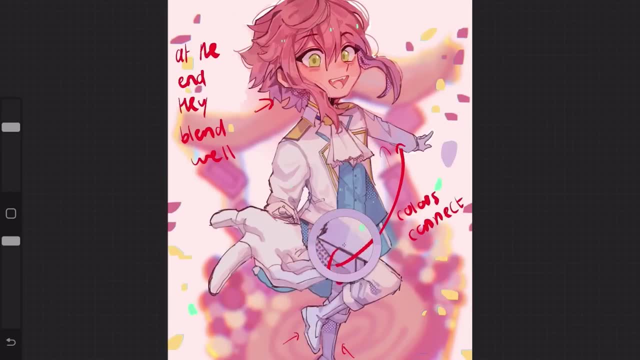 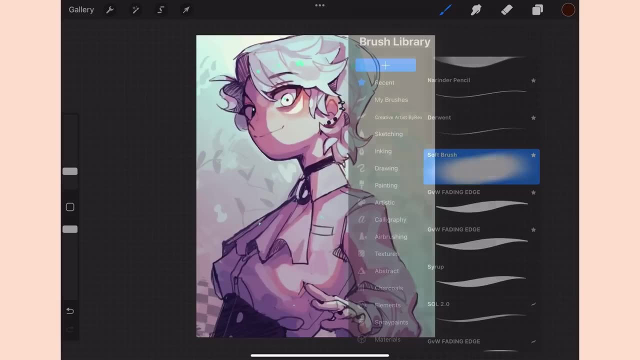 you like, visualize it. so I don't just use gradients on a small scale, I use gradients for a whole piece. it's a great way to add values that blend into each other, like, for example, this piece on this area is a blue and then the gradients into purple. I did this with layers and layer blending modes, but the 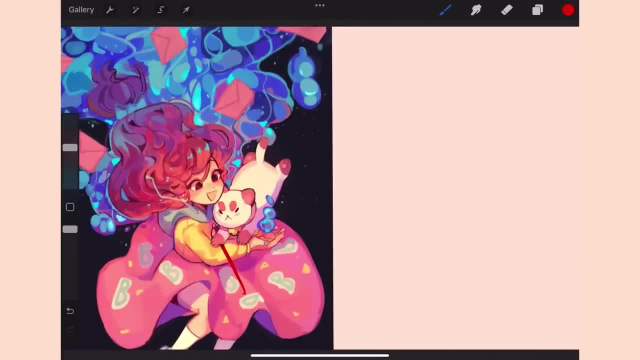 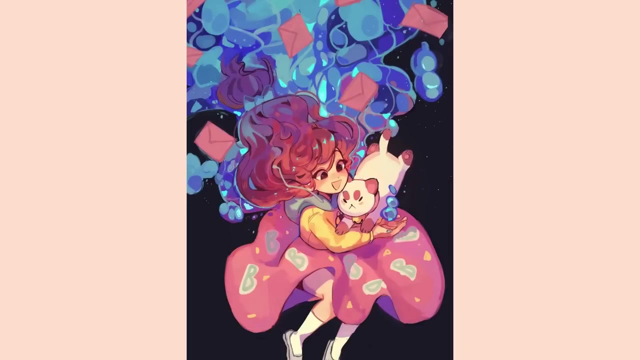 basic idea is this: this piece is my favorite gradients I've ever done. there are two gradient shifts here: one from the figure, which is yellow and purple, and the one in the background, which is dark blue, and the other one from the blue to light blue. these colors also contrast each other, so B pops against the background along with 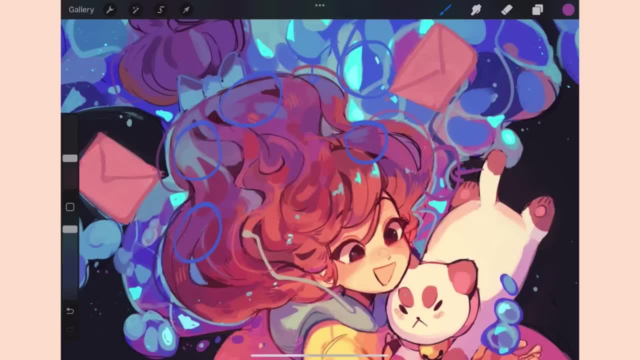 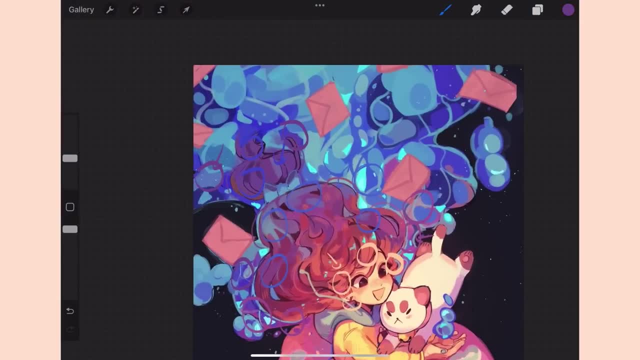 her still having hints of the background color in there. so the blending I was talking about earlier, you can tell I've blended in the blue into the hair and I've also blended the purple of the hair into the blue color. it just kind of like helps the piece. 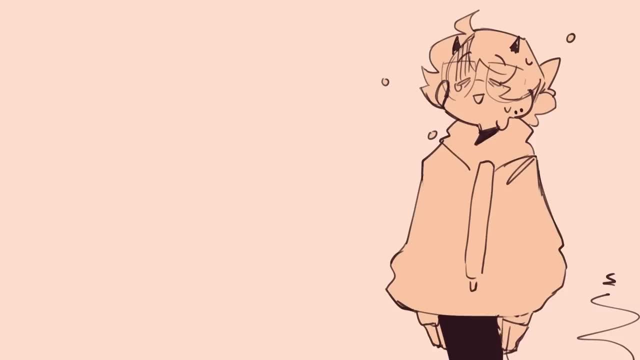 mush together but not look too muddy. make use of the layer opacity for shading, lighting and adding random hues. this is great for gradients effect I was talking about. this is the bare basic process to picking colors for me. I will show you an example of a process here and touch on sections I think are 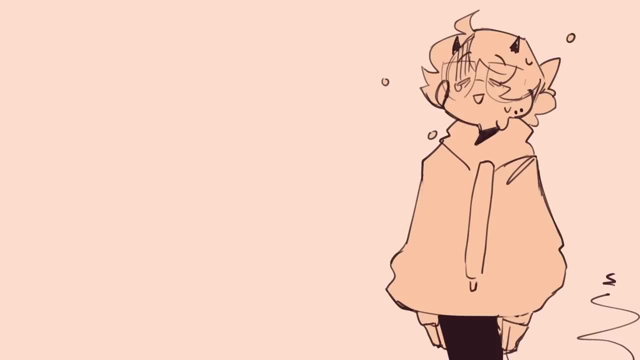 important to have a visual representation. I cannot teach you straight-up picking colors. I wish that was that easy, but it's something you have to put in the work and get better at. with time and effort, you'll be able to understand colors well enough to be able to place them into a piece and have a good result. 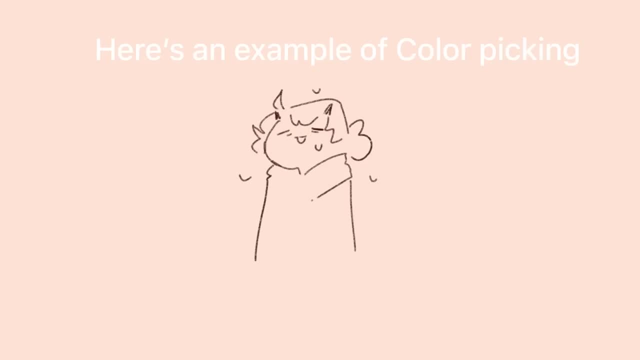 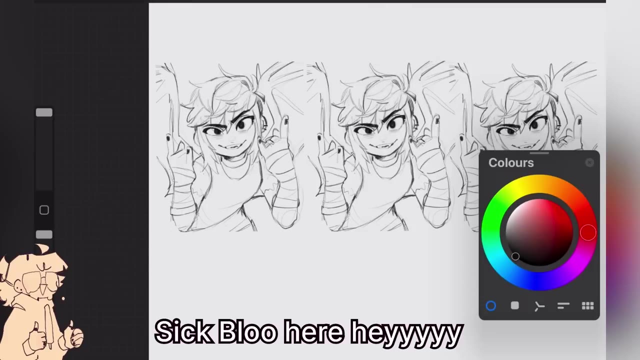 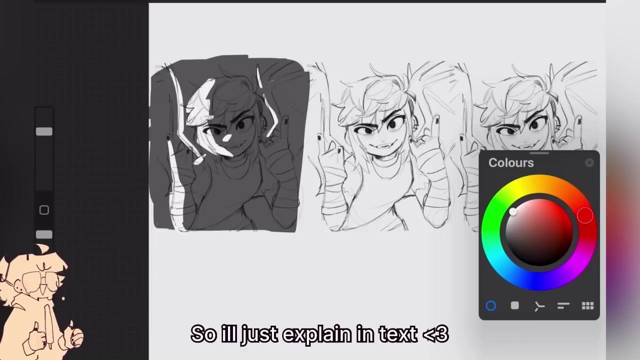 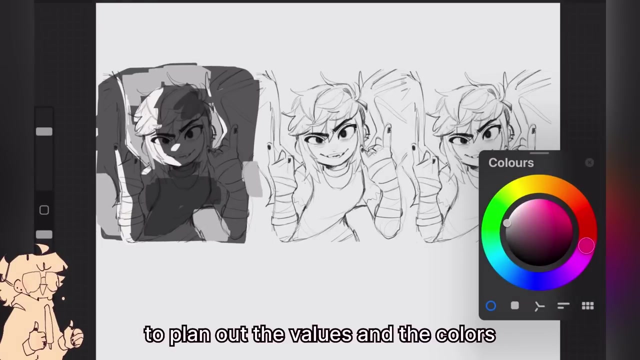 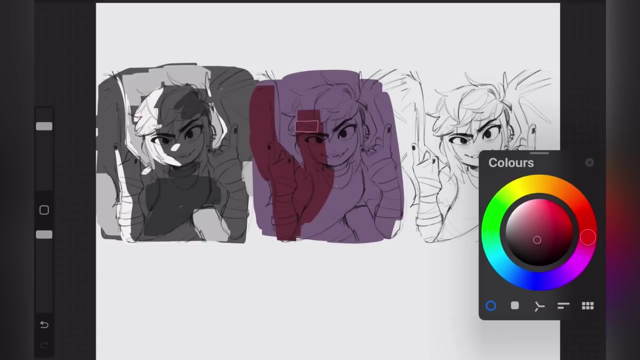 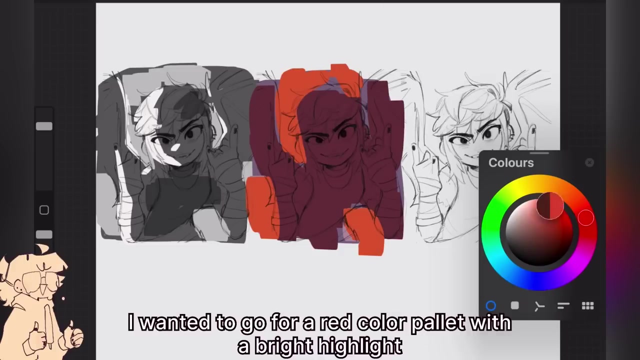 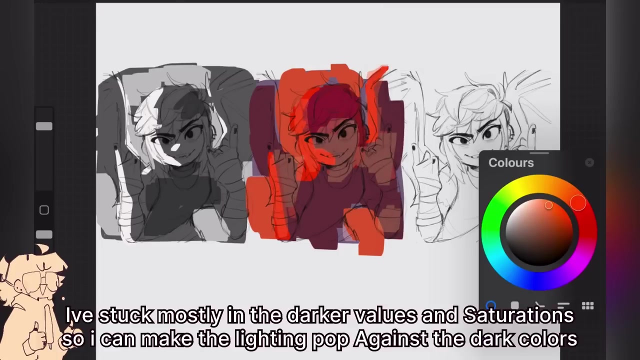 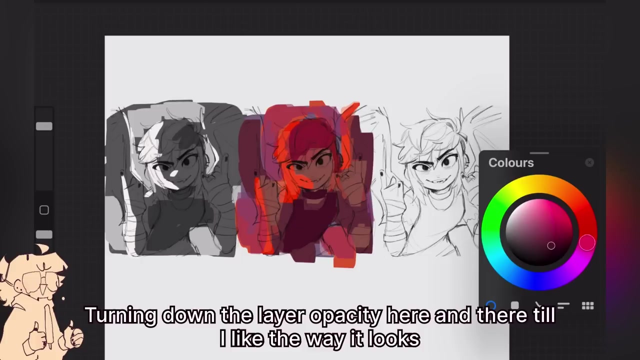 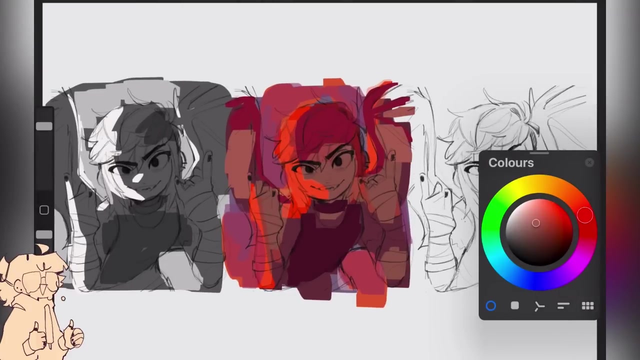 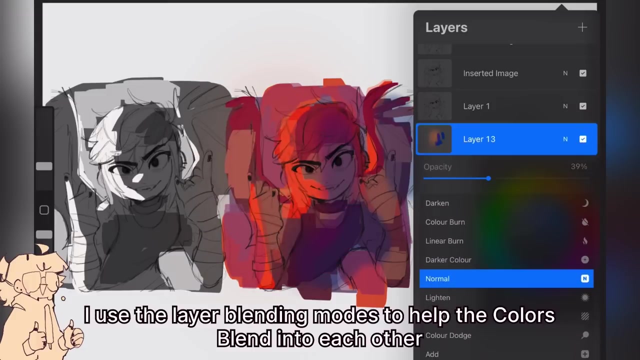 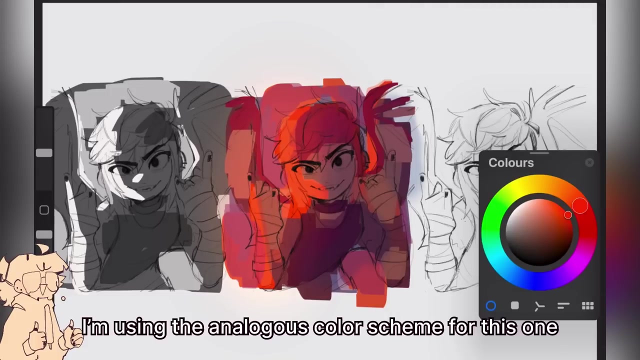 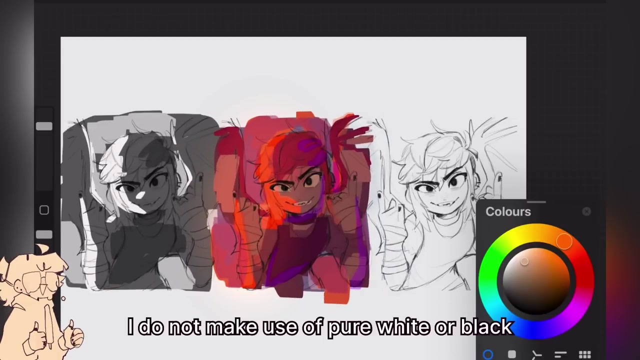 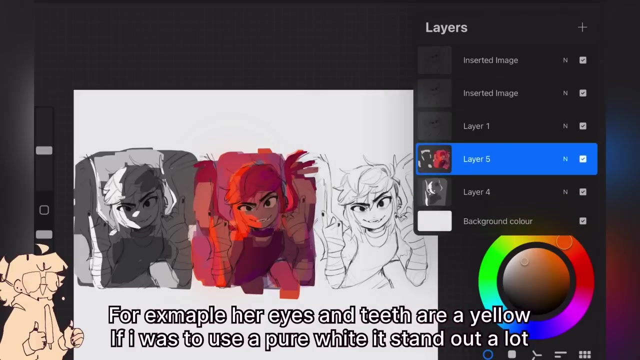 understanding of color theory, because those colors are Northeast and apart from being in North защ施 チーズ, Combo, Zipper, Toenail, Chiffon, Wooden, Sennit, Bitch, Scissors, 먼지, Persimmon 手. Thank you, Thank you. 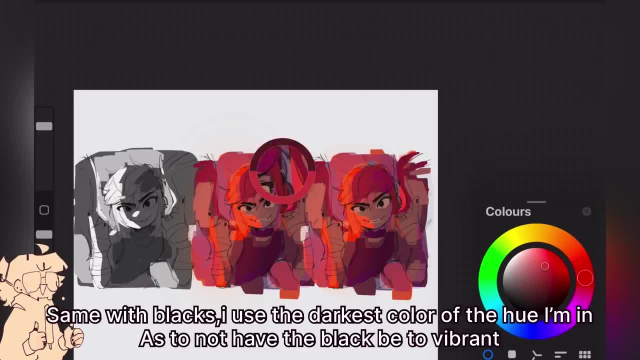 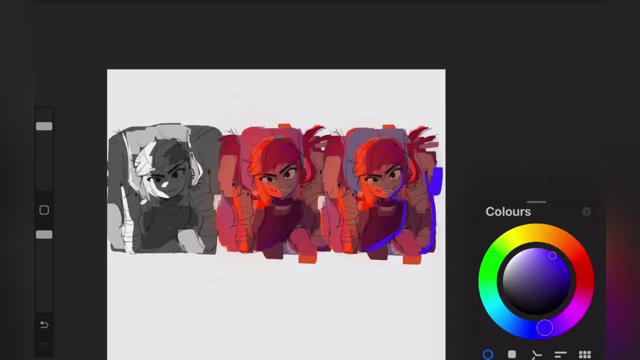 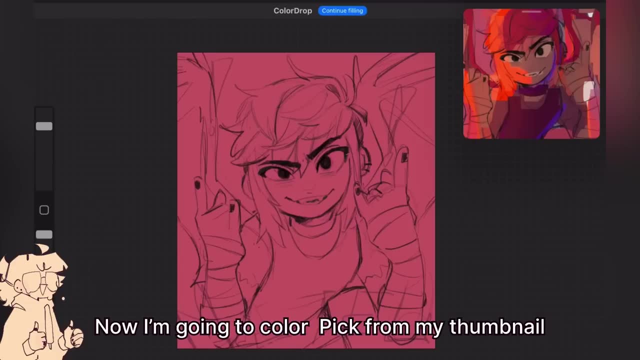 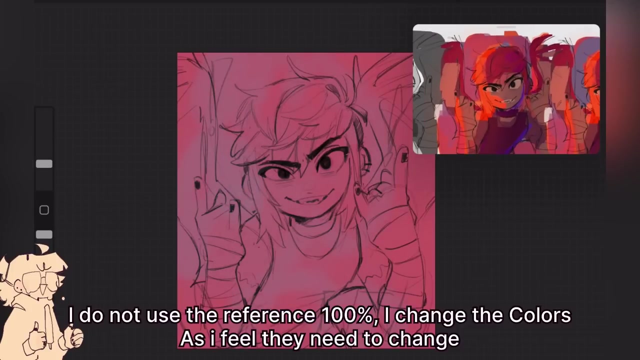 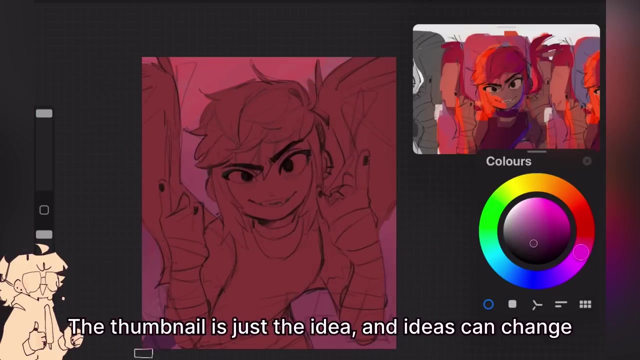 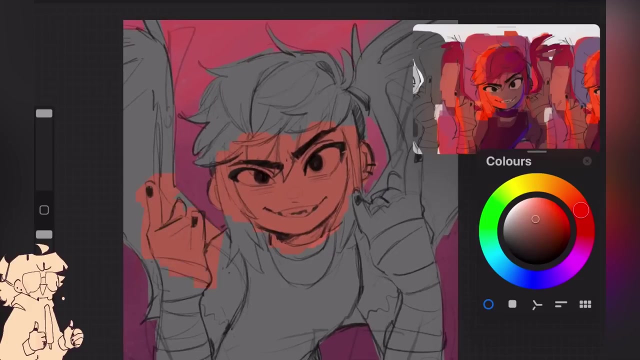 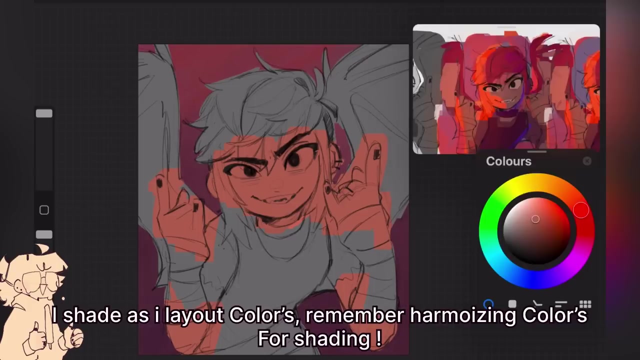 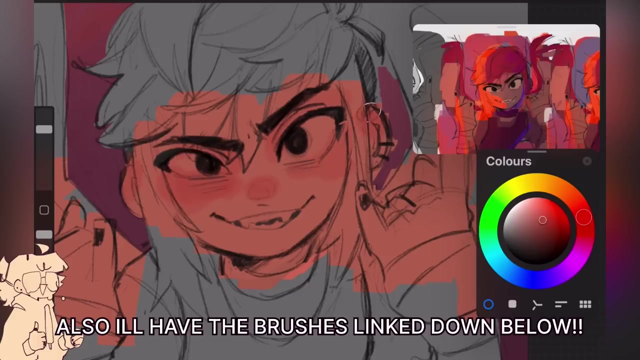 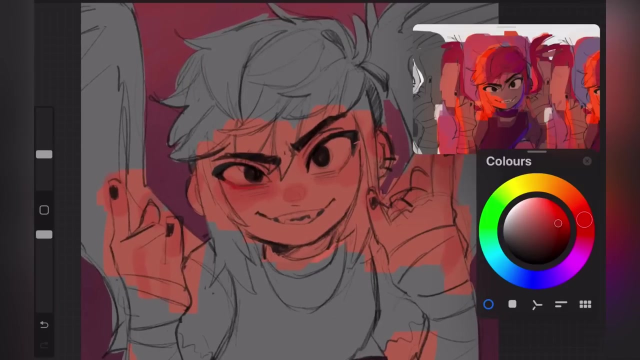 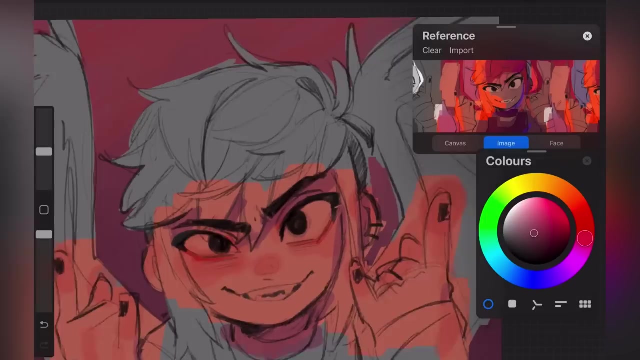 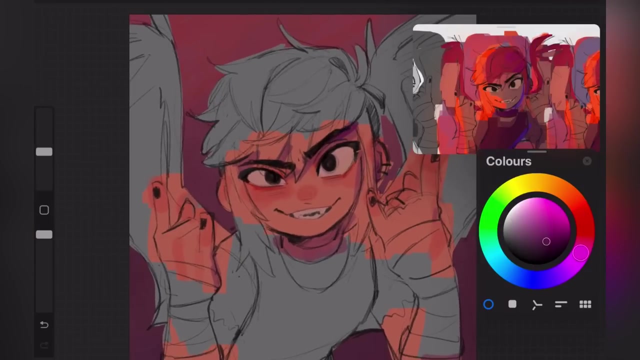 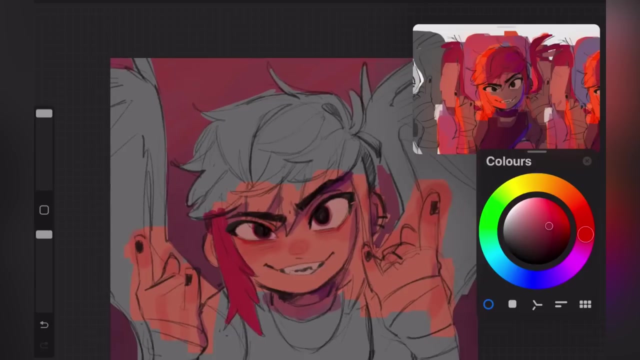 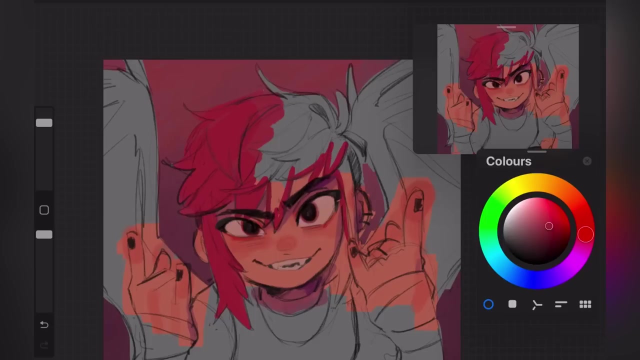 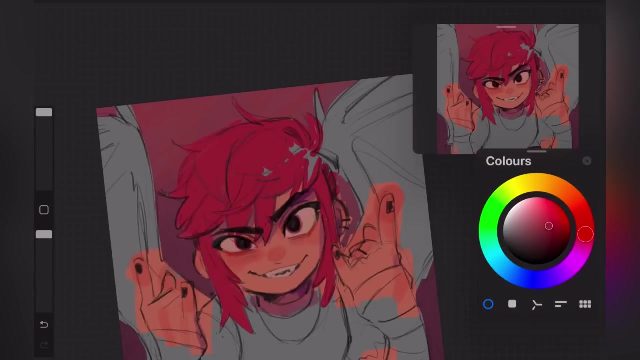 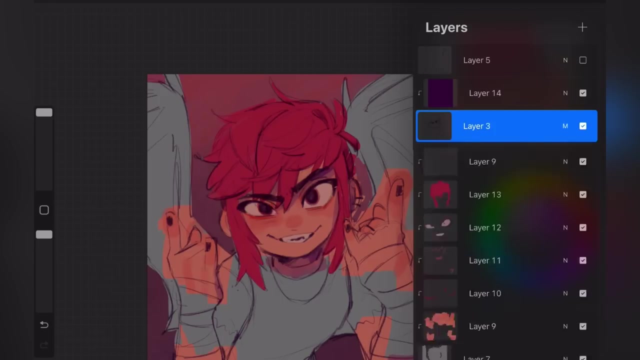 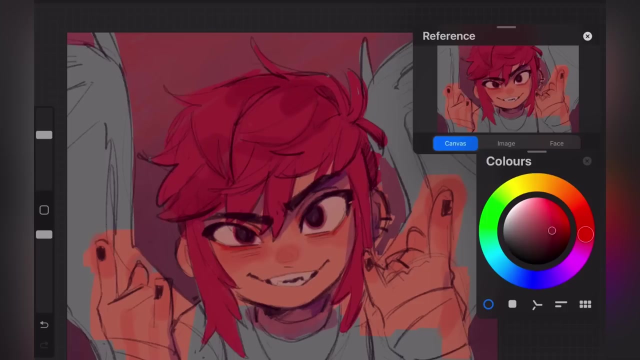 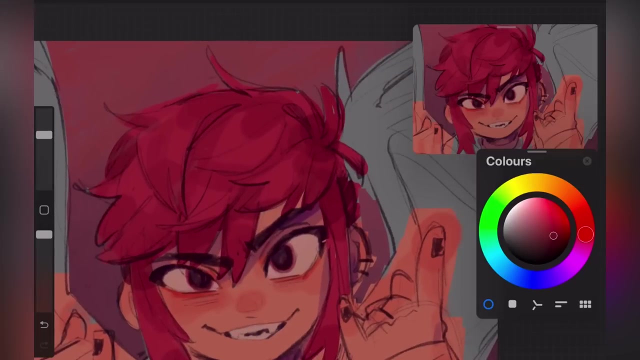 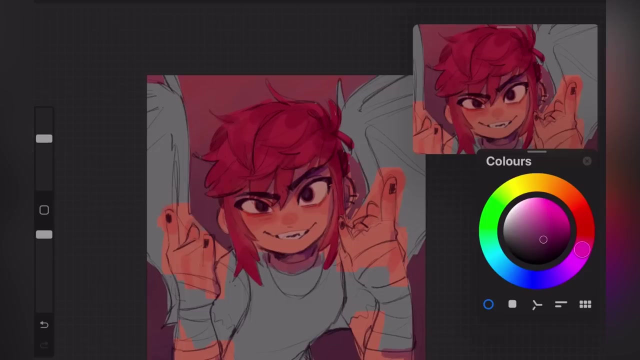 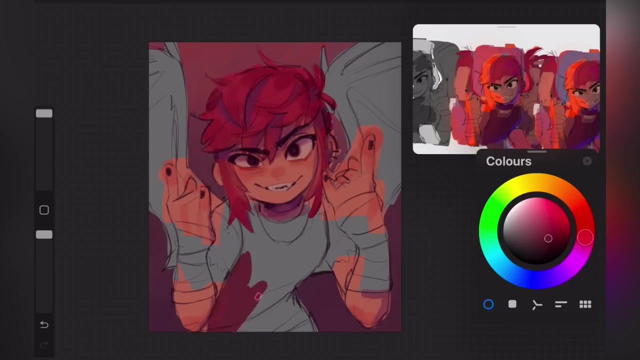 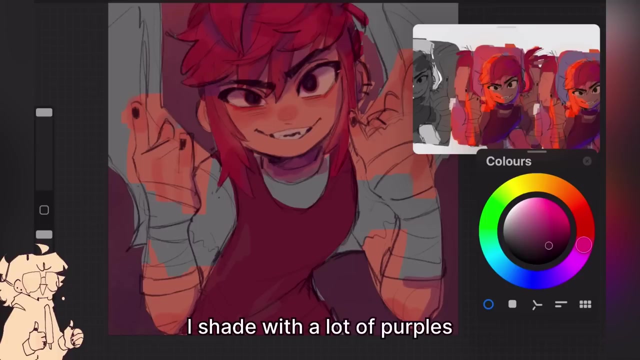 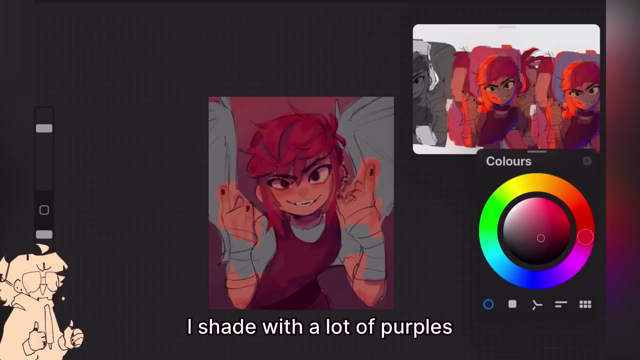 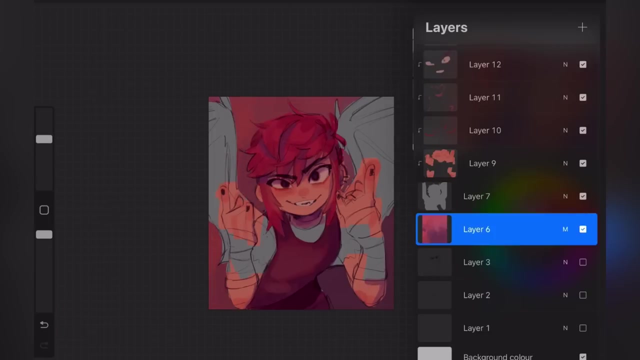 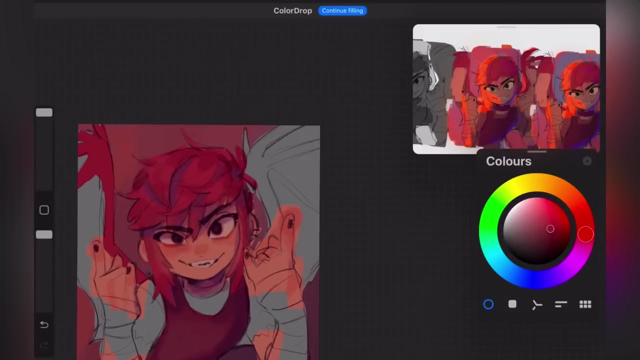 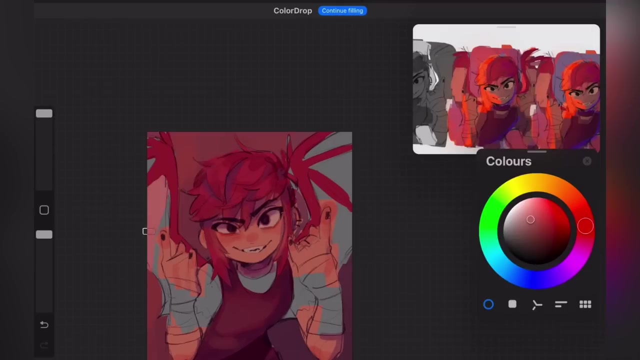 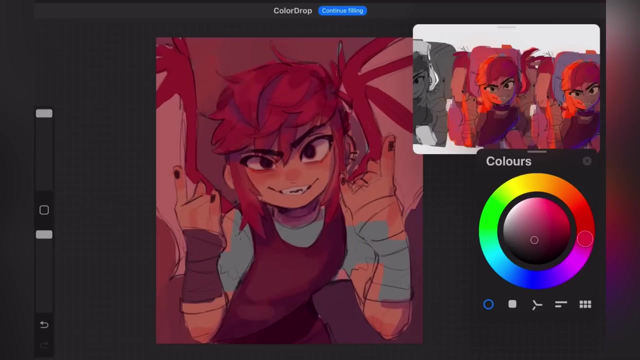 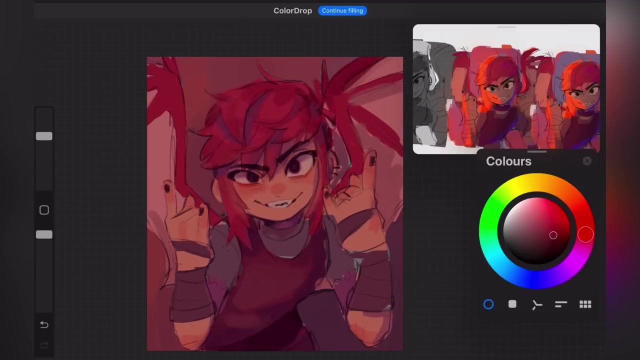 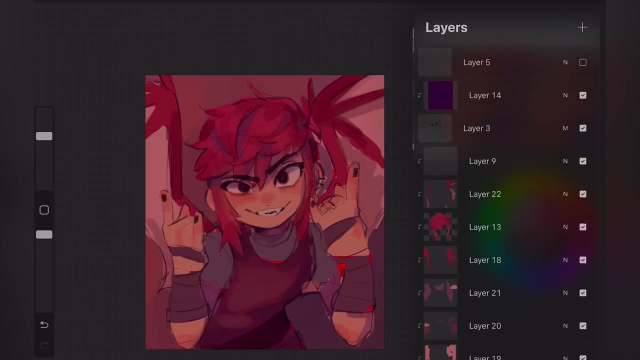 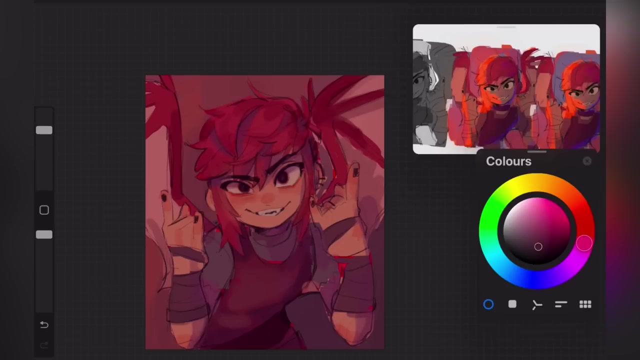 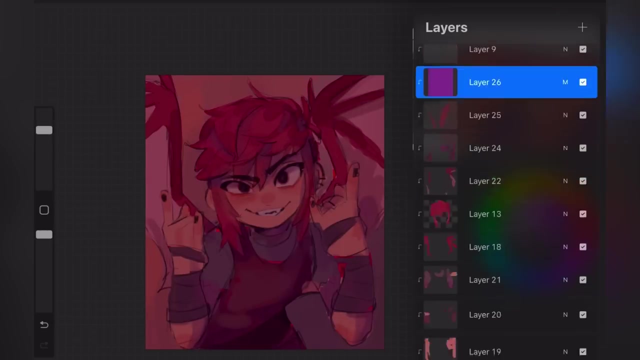 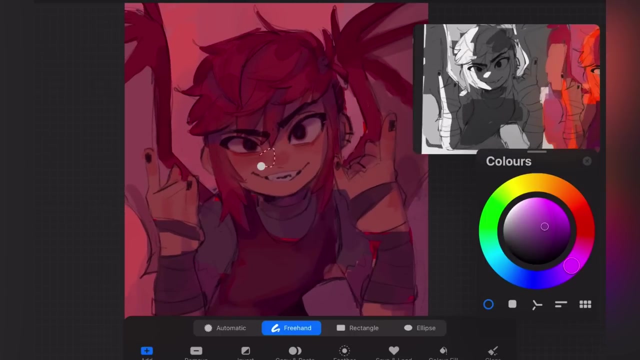 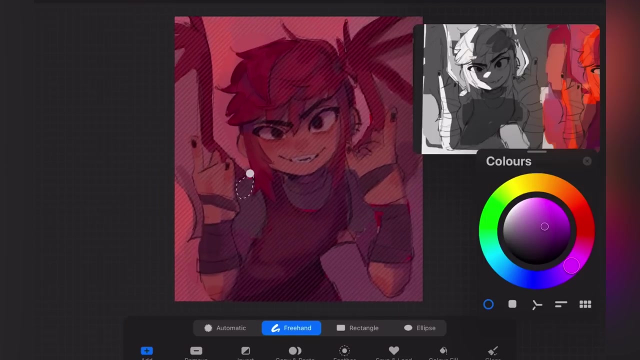 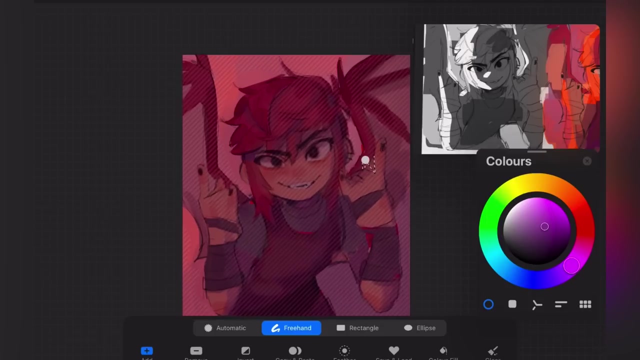 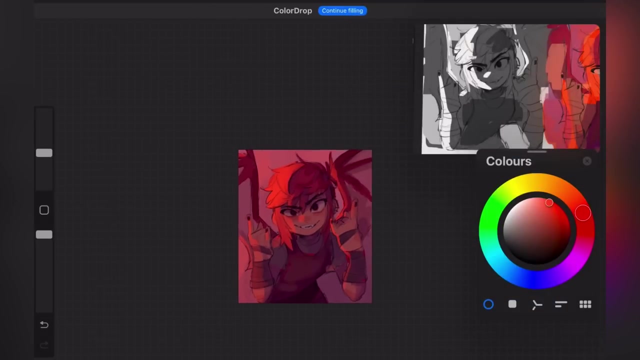 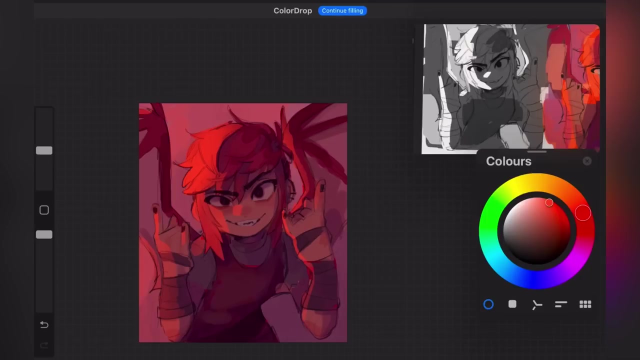 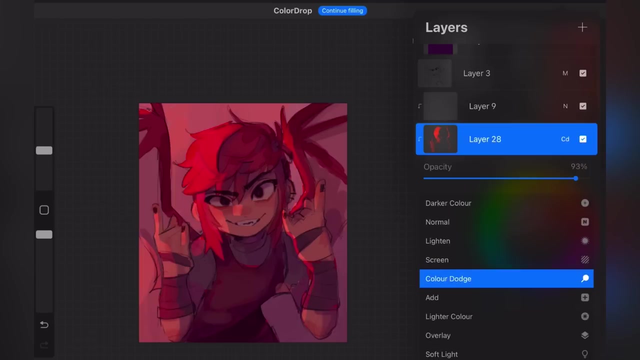 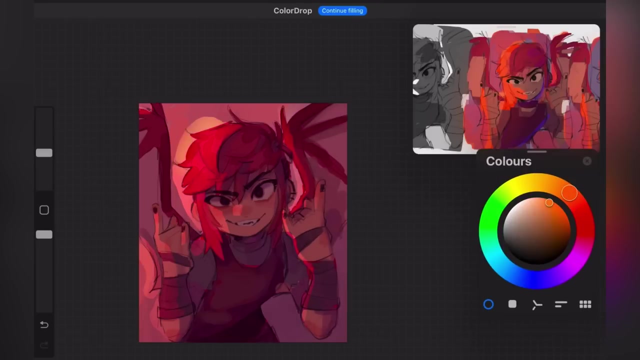 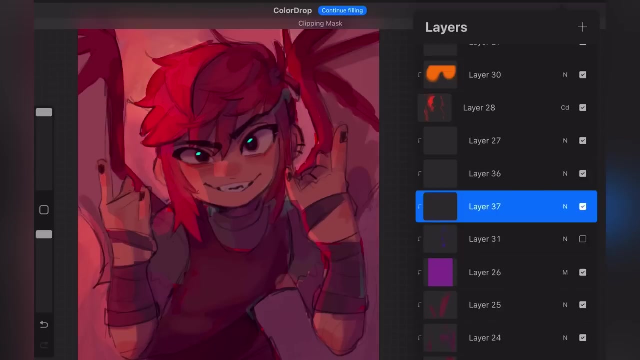 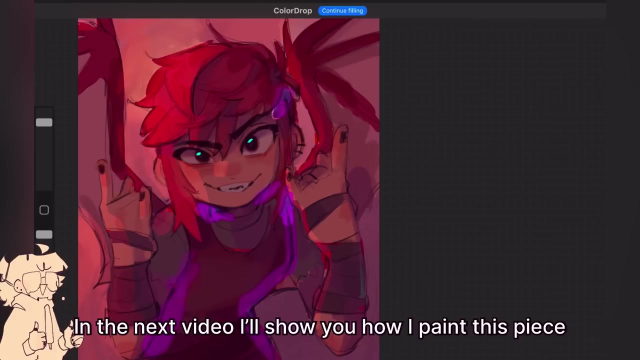 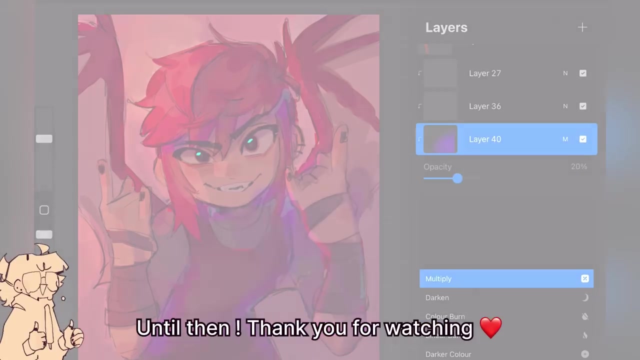